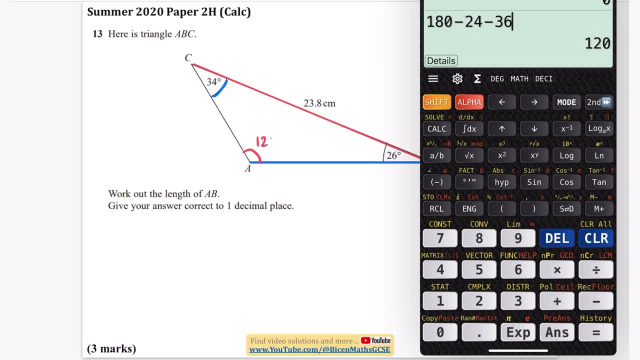 180,, take away 24, take away 36.. So I'll do 180,, take away 24,, take away 36.. So I'll do 180,, take away 36, and that angle is 120 degrees. So this 26 degrees, because it hasn't got anything, that's. 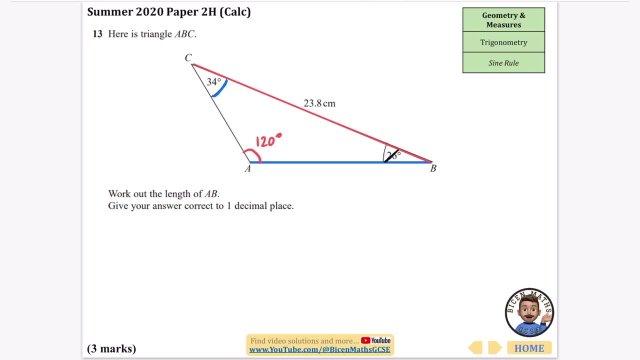 opposite it. I'm actually not going to be using that at all, okay. So I'll just leave kind of a line through that saying I don't need to use this So to do the sine rule. I'm going to say that my 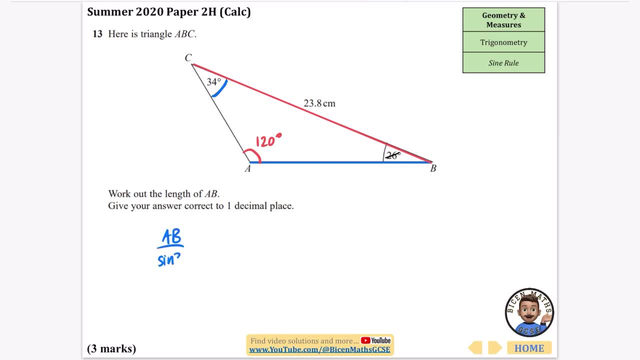 AB. the length that I'm looking for divided by the sine of 34, is equal to this other pair, So it's going to be this one divided by the sine of that. So that's going to be the sine, sorry. 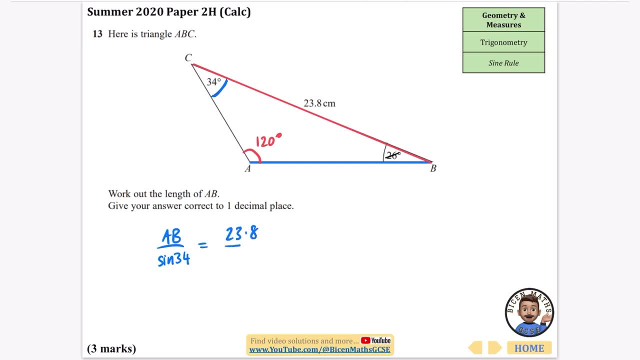 not the sine, that is going to be 23.8, divided by the sine of 120.. And you know what? I'm going to make that in red, so that it's the right colour that matches with what's on the diagram. Now, if I want to find out what AB is, 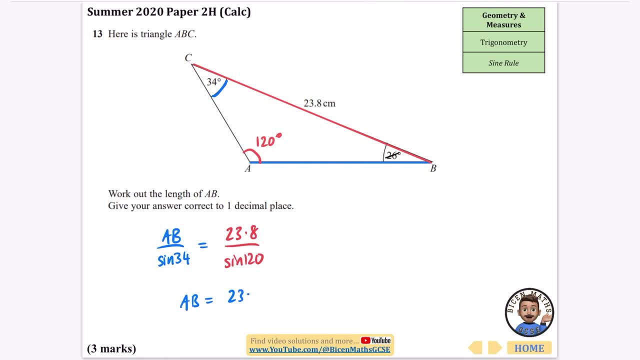 equal to. I'm simply going to multiply by sine of 34.. So that's 23.8 divided by the sine of 120, and I'm going to multiply that by sine 34 and get it all typed in to the calculator. So slide my. 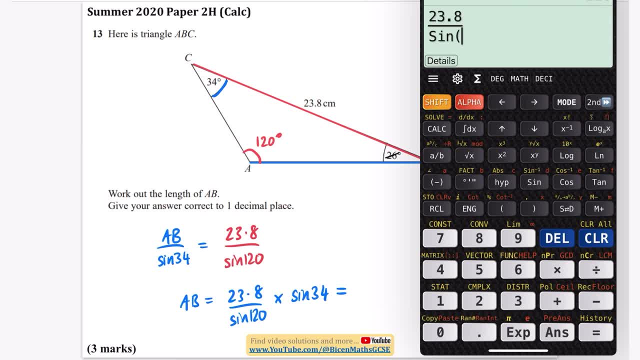 calculator back in. I'm going to get 23.8 over the sine of 120, multiplied by the sine of 34, and I get the answer to one decimal place of 15.4 centimetres. 15.4 centimetres for this one. 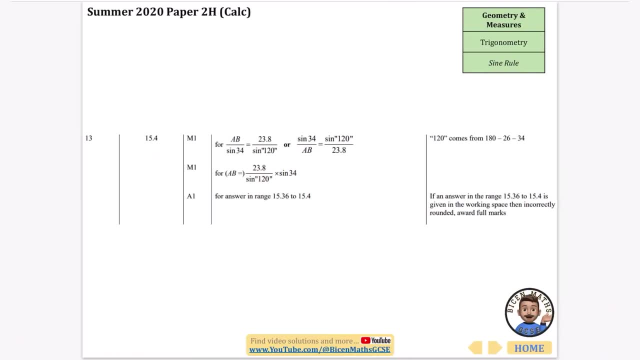 Let's double check to see that we've got this one correct. There is the 15.4, and it was a pretty straightforward one because it was only a three marker. Now this one actually says sine rule, but I will have changed this by the time you go to download this. This isn't going to be sine rule. 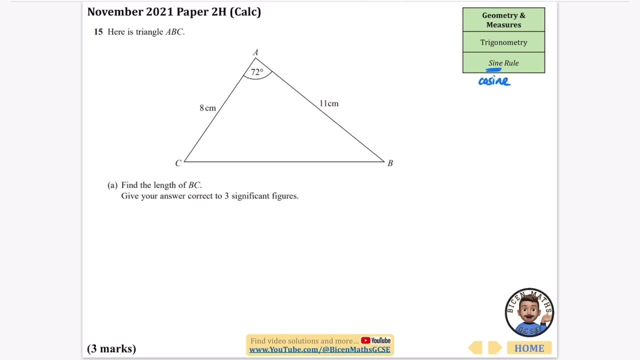 This is actually an example of a cosine rule, And the one that we're looking for here is BC. Now, because BC, we- and we- sorry, because we are looking for BC- also know the length of AC and we know the length of AB as well, then this means we can. 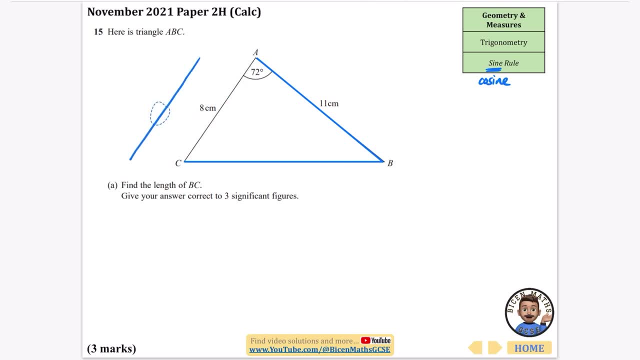 actually use the cosine rule. I'm just going to do that one, so it's a straight line as well. make it look nice and neat. And we know this angle that is opposite over here, which is 72. So I'm going to say that this side, which is opposite, sometimes people like to call this like 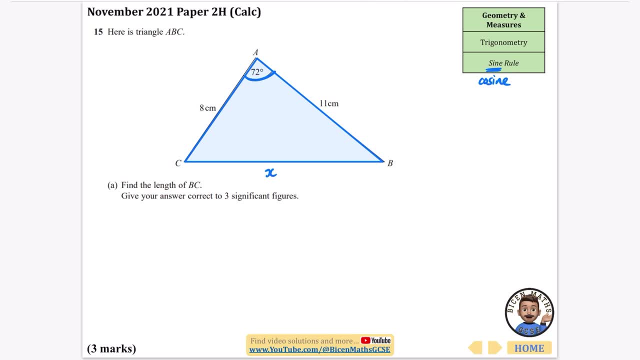 X or sorry, like they like to call it X, but I'm actually going to call it just BC in this question. Now, the cosine rule is this: that A squared plus- sorry- B squared equals B squared plus C squared, a bit like Pythagoras minus 2BC. cos of A. 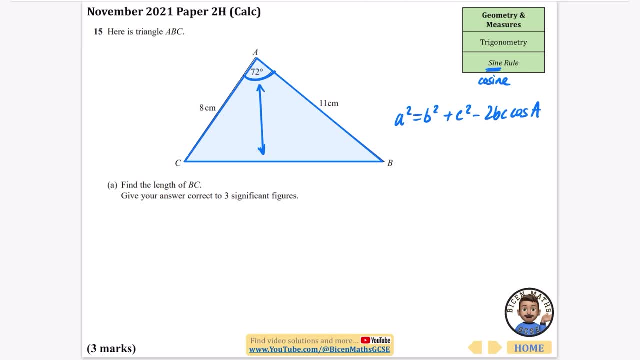 So the key thing is that the side you're looking for has to have an angle that is opposite. So in our case, our A squared is this length that we're looking for BC squared, And that is going to be equal to the 8 squared plus the 11 squared minus 2 times 8 times 11,. 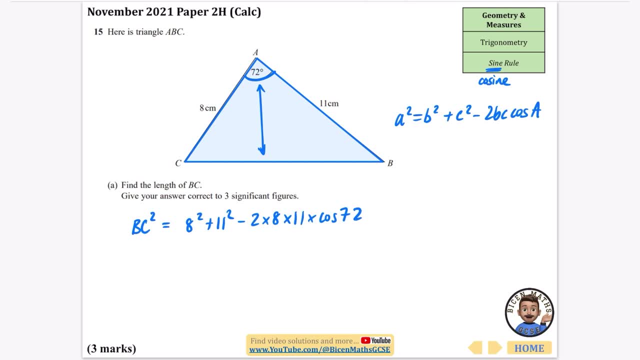 multiplied by the cos of the angle that is between them. So this B and C that we have here, the angle which is capital A is in between these ones that we've got, So I try not to really remember it as this formula. 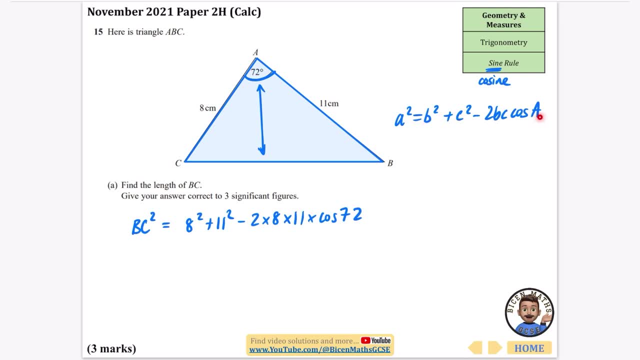 I try and remember it, as all of this stuff is talking about two sides and the angle between And this is the angle that is opposite. So if I want to find out what B-C is equal to, I am literally just going to do the square roots of what I've got there. 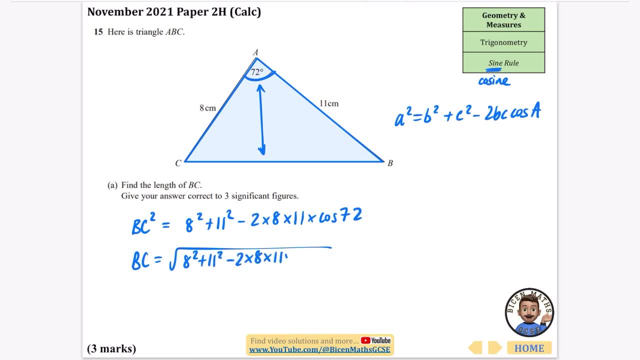 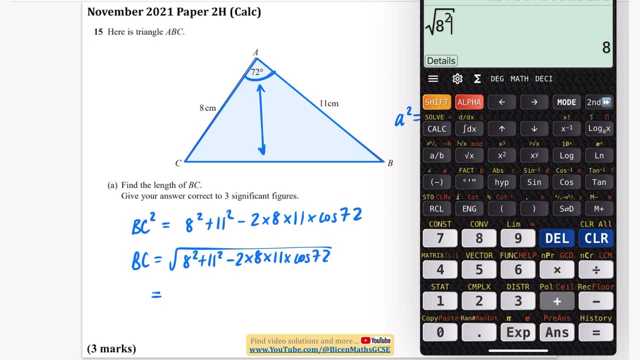 So that's my 8 squared plus 11 squared, minus 2 times 8, times 11, times the cos of 72, and that's going to tell me what B-C is equal to. So square root of 8 squared plus 11 squared: 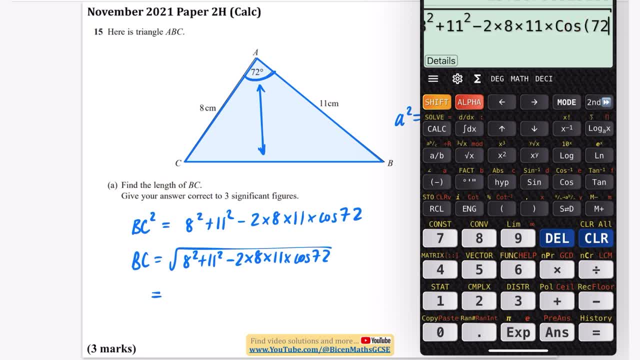 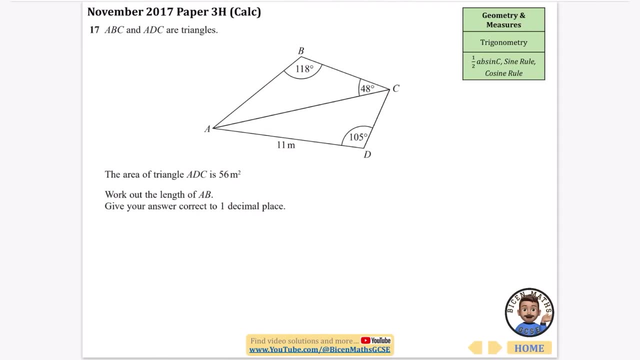 minus 2 times 8 times 11 times the cos of 72, it's already done the square rooting. so to three significant figures, it is 11.4 centimetres to three significant figures. Let's double check. we've got this one right. yep, there is the 11.4, so we know we have this one correct. This is now where we start doing. 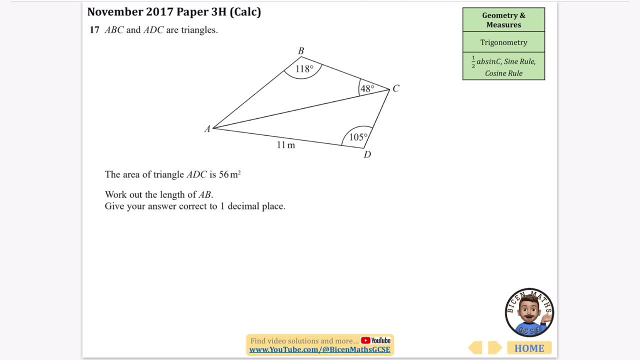 a mixture of different kinds of things. we've got two triangles that are stuck together. we've got all the information on here. the thing that I think we're going to start off with is that the area of triangle ADC is 56, so this one that we've got here has an area of 56. so if we use the half AB, 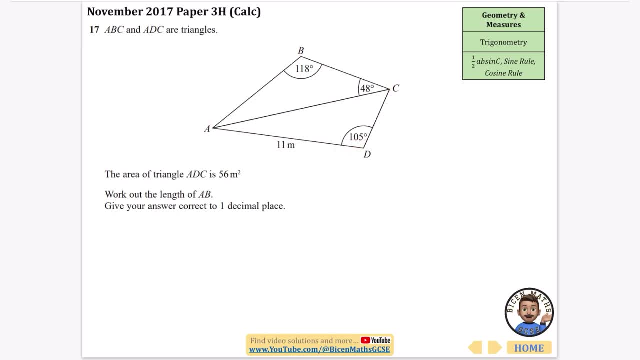 sine half AB sine C rule. I can see that I have got a side and I have an angle and I'm going to try and find out what the other side is using a half AB sine C. So, because I know that the area is 56. 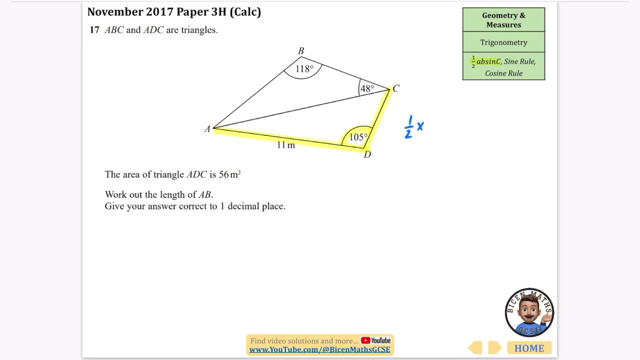 I can say that a half multiplied by 11 multiplied, I could call this x as a side, but I'm actually just going to name it what it is: multiplied By CD, multiplied by the sine of 105, that's my half. AB sine C, that is equal to 56.. I'm going to use 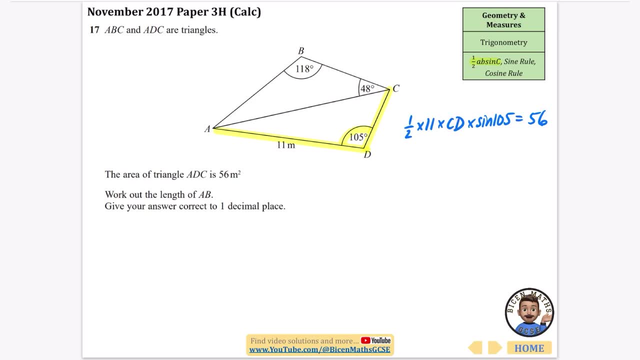 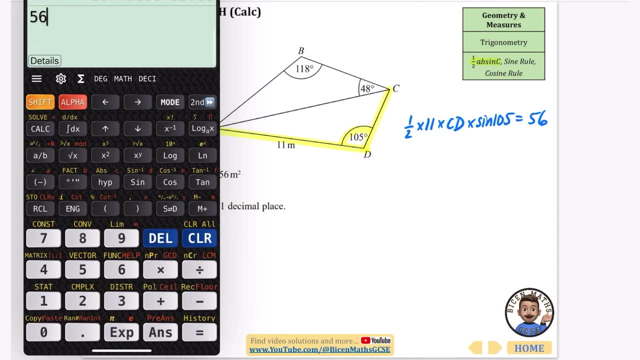 this to find out what CD is. CD is literally just a length. so what I can do is I can do 56 divided by these three things that we've got here. So on the other side of the page I'm going to put my calculator, I'm going to do 56, I am going to divide it by a half to get rid of the half. I'm also going 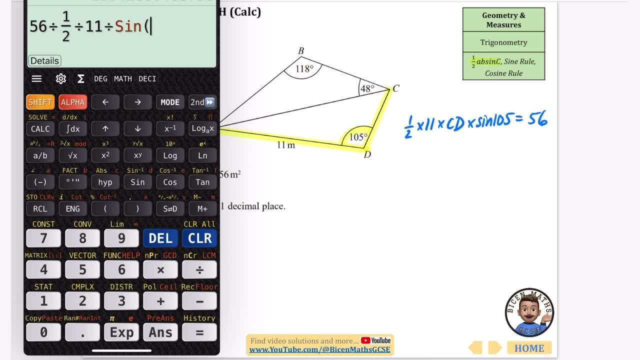 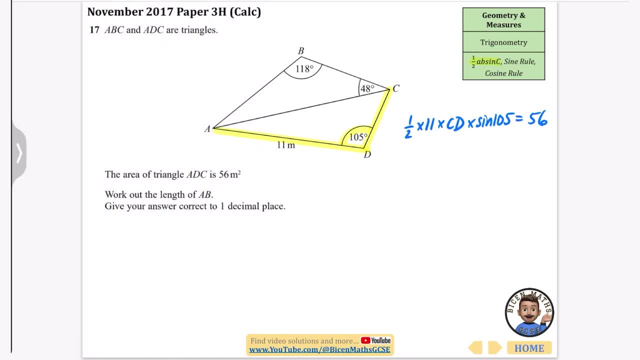 to divide it by the 11.. I'm also going to divide it by the sine of 105, which tells me that the length of CD is 10.541, 10.541, and the reason I'm doing a few extra decimal places here is because at the end it 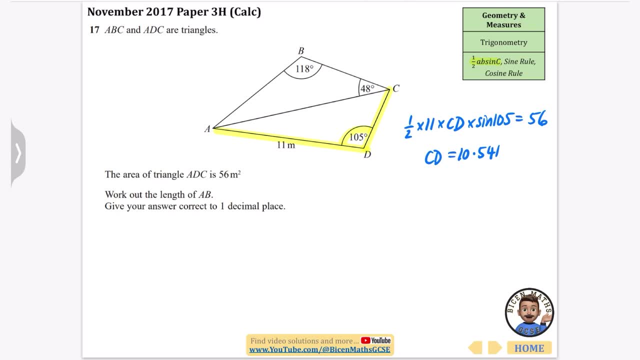 wants it to one decimal place, so I have a bit more detail as we go. it'll probably mean I have a good level of accuracy as we go. So that is 10.541. is this length that I have just worked out here, and the thing we're trying to find out is the length of. 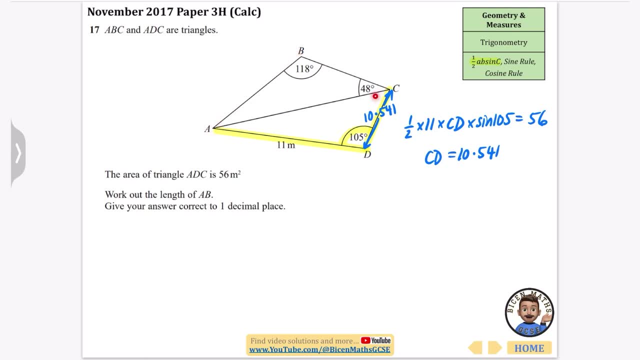 AB that we've got. Well, I think this side of the triangle is probably going to help, because once I get this side of the triangle, I've then got a separate triangle that I can do some calculations with. So this triangle that we're going to look at now I have got my AD and my C. I know that this 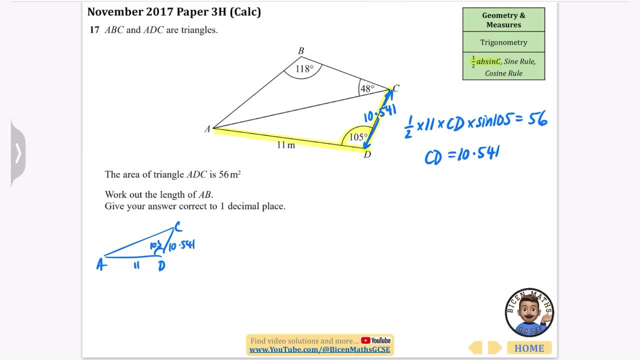 is my 10.541, this is 11 and this is 105, so I can use the cosine rule on this particular one that I've got. So I'm now going to use the cosine rule, which means that, AC squared, the opposite side is going to be my 11 squared plus my 15 squared. So that's going to be my 10.541 and that's going to. 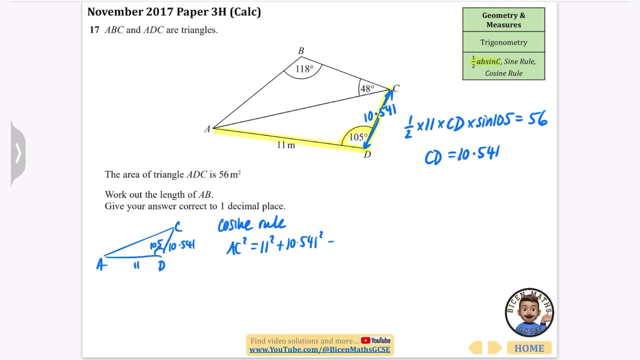 be my 10.541 squared, that's my A squared plus B squared, minus 2 times A, times B, times by the cos, because it's the cosine rule times by the cos of 105.. Now I'm going to put that all on the calculator. 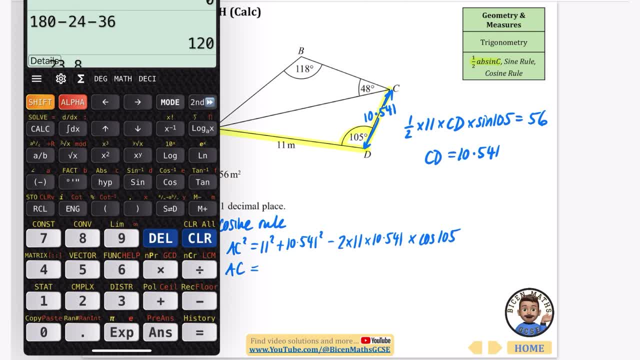 with the square root sign, but I'll save myself a bit of writing out. So I'm going to do the square root of the square root of 11, squared plus now. that's previously stored in my calculator as the answer, So I'm actually not even going to bother typing that in. I'm actually just going to write. 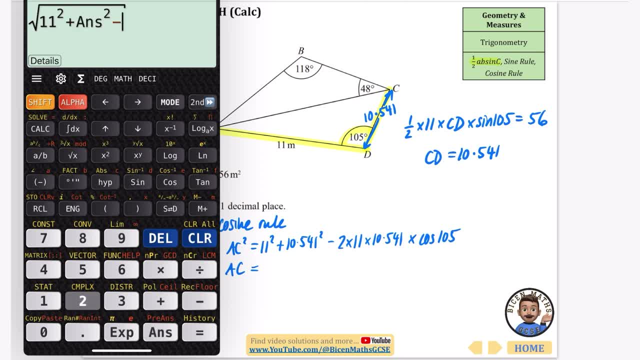 plus the answer squared, the calculator knows what we're doing- minus 2 times 11 times the answer times by the cos of 105.. So every time I've typed in answer, the calculator knows that I'm doing the 10.541.. So this tells me that the length of AC is 17.0919, etc. like this. Now I know how long. 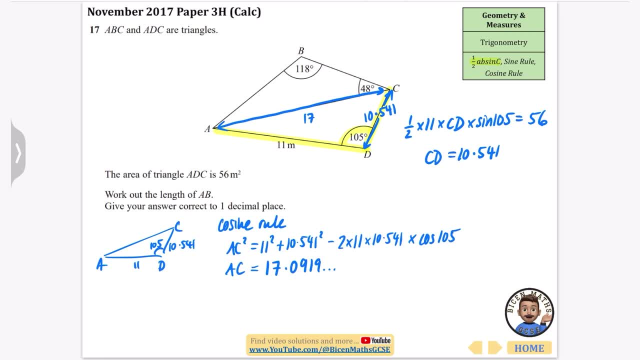 this part of the triangle is, it is 17.0919.. So we're going to now see if we can figure out the length of AB, and that's actually going to be a straightforward sign rule, because I've got these two, which are a pair, and then I've got these two. 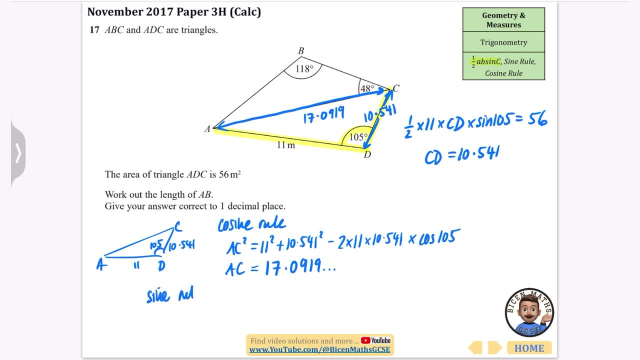 which are a pair. So my last part is to do the sign rule, and the sign rule is that AB divided by the sine of 148 is going to be equal to AC, which is 17.0919 divided by the sine of 118.. So this thing, 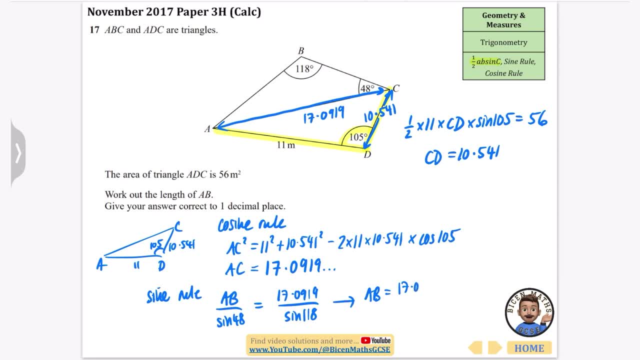 tells me that AB is going to be equal to AC divided by the sine of 118.. So this thing tells me that AB is going to be equal to 17.0919 divided by the sine of 118, multiplied by the sine of 48.. And I'm just going. 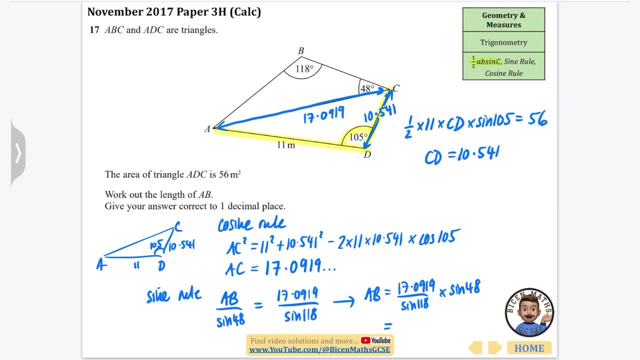 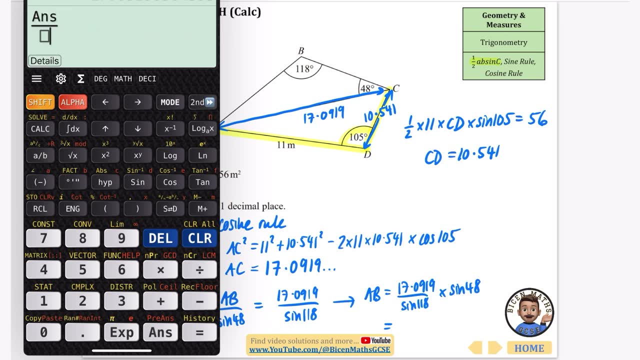 to put that all in my calculator. Remember though, this is already stored as my answer, so I can type: answer divided by this times this. So there is my answer. I'm going to do the answer divided by the sine of 118 and I'm going to multiply that by the sine of 48.. We come up that A is 14.4 to one. 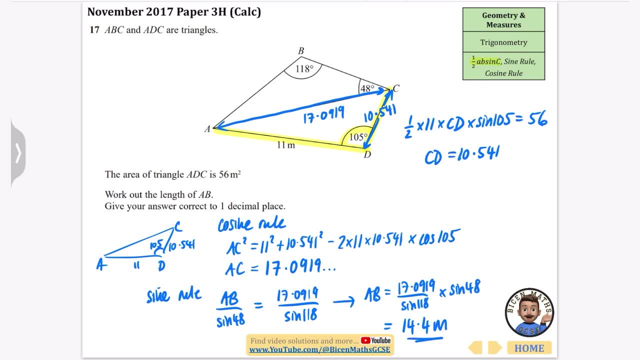 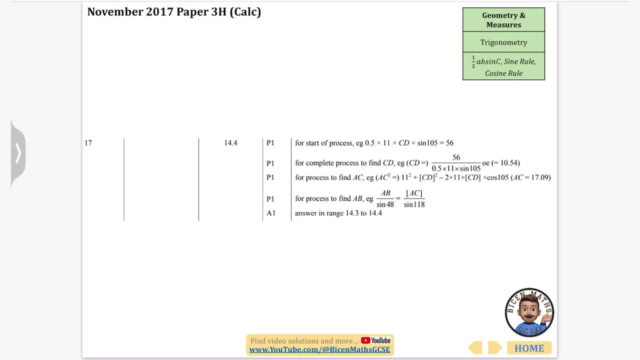 we get that AB is 14.4 meters. Let's see if we've got this one right. There is the 14.4 and you can see in here the process of doing the half AB sine C, and then we've got some bits here with the cosine. 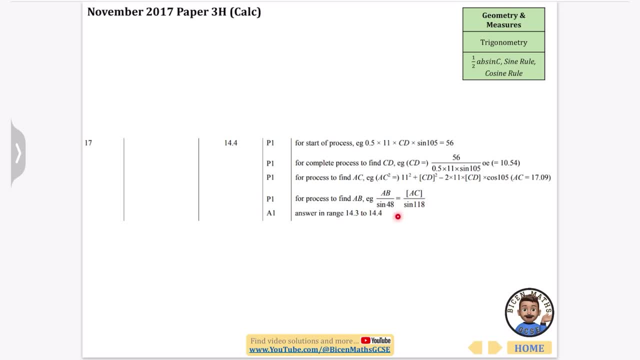 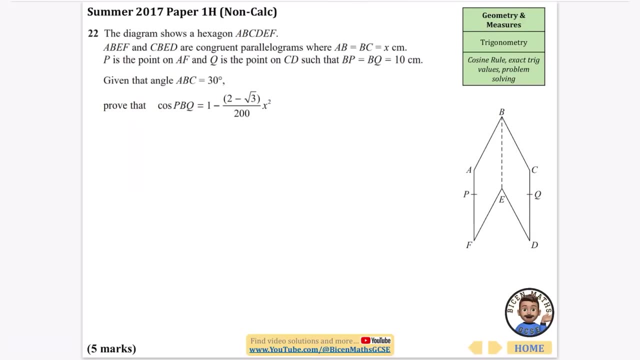 rule and then the sine rule, They would have accepted 14.3 to 14.4.. Okay, I'm going to put the calculator back to the other side, where I usually keep it, and now we're going to look at this next question, which is pretty tough, if I'm honest. So it's going to be a mixture of the cosine rule. 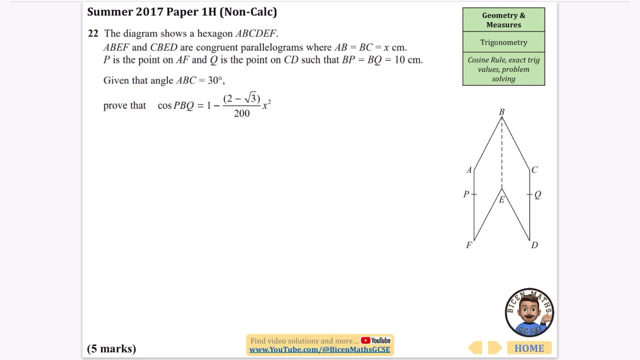 exact trig values, problem solving, and it's a non-calculator one, which is why I've said exact trig values. The diagram shows a hexagon. ABCDEF, ABEF and CBED are congruent parallelograms where AB is equal to BC, which is equal to X. So I'm actually just going to label that, those two. 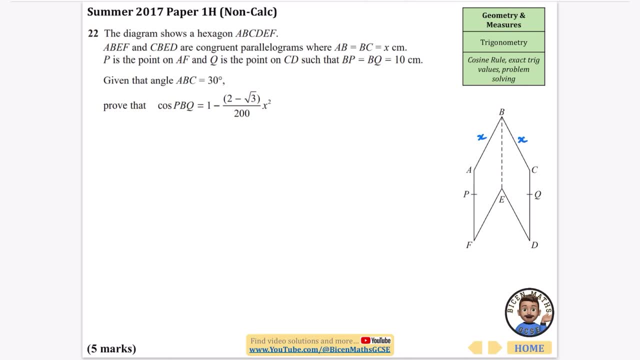 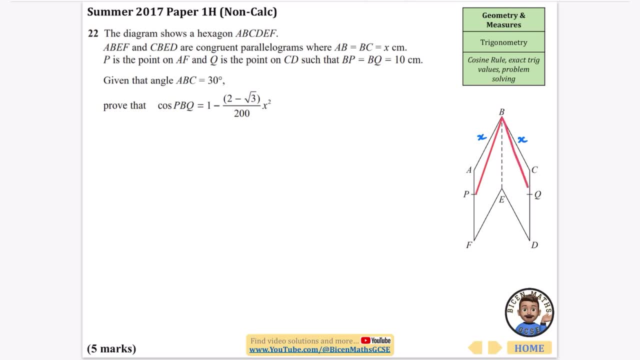 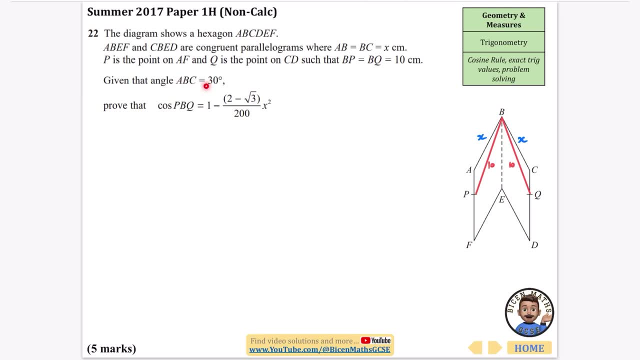 and it says: given that angle ABC is 30, so I'm going to say that this whole angle that we've got at the top is 30. so I'm doing that one in blue, and it wants us to prove that the cos of PBQ is equal to this thing that we've got here. Well, this is very, very tough. I'm going to show that. 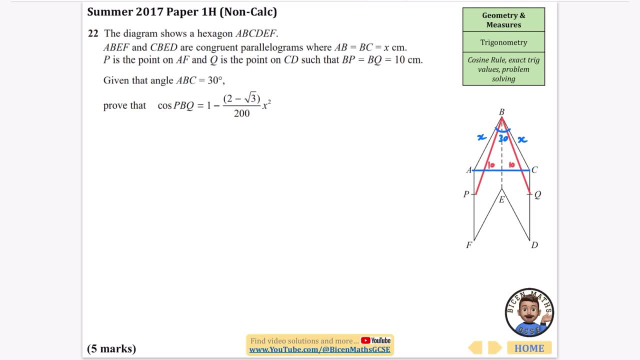 AC. I know something about AC and PQ. AC and PQ are the same length as each other, which means I've actually kind of got like two triangles between this. but I'm wondering if it's going to fill that in for me. I don't really. 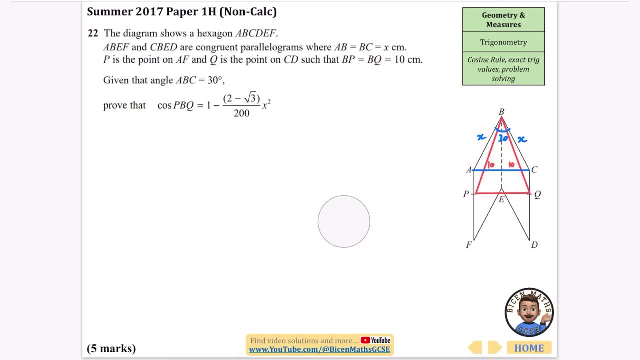 want it to. Let me just see if I can remove that area. Perfect. So we have got two different triangles and I'm going to draw them out separately and then we're going to do some maths with this. So the first one is the blue triangle, and the blue triangle is with A, B and C, where this is X, X. 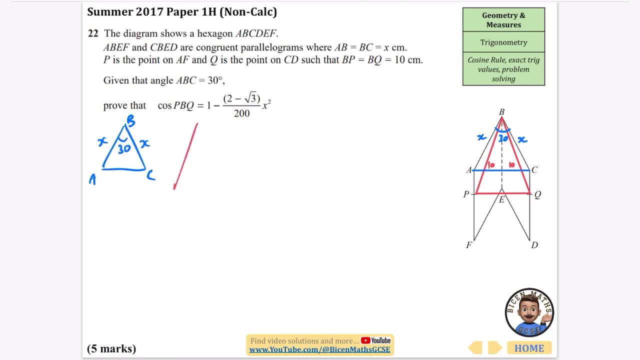 and 30, and then the second triangle that we've got, which is a bit longer. it looks like this, where we have P, Q and B. This is the angle that I'm interested in. at the top, This is cos of PBQ. This is the one that I'm talking about right here, and we also know that this length is 10. 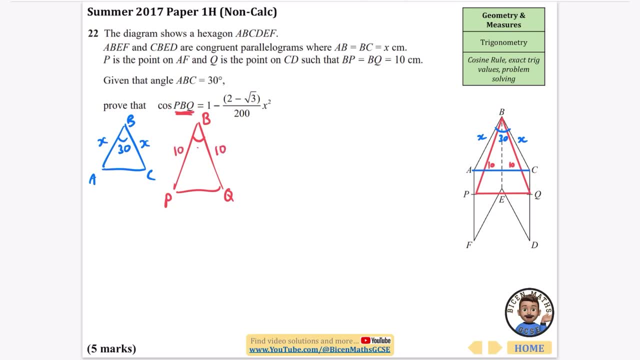 and this length is 10.. Something else that's pretty important about this is that this length is equal to this length because of just looking at the diagram. They must be, because they're going from one side of the parallelogram to the other side of the 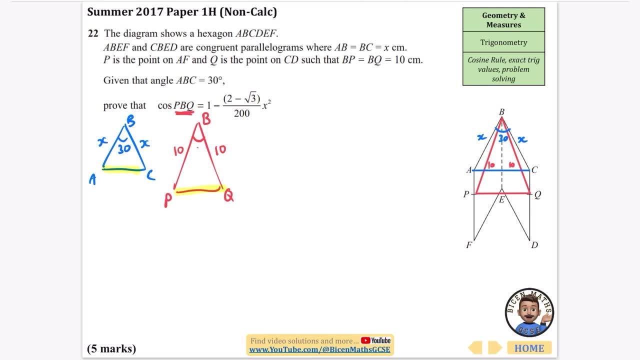 the other parallelogram I should say- So I'm just going to do a little side note- that AC is equal to PQ. I'm going to do the working out of the cosine rule for this blue triangle that we've got here, So I need enough space for this. We're going to do the cosine rule and the cosine. 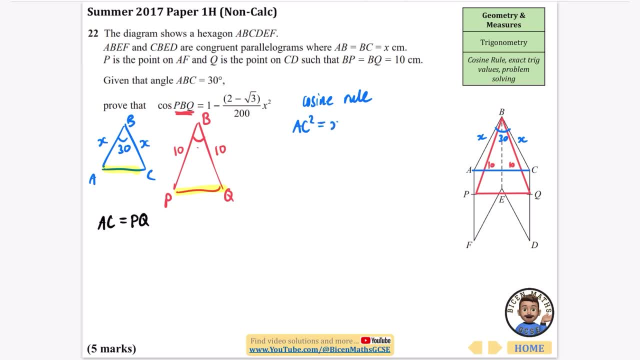 rule will say that AC squared is going to be equal to that side squared plus that side squared, So that looks like Pythagoras. and then you do minus two times these sides together, minus two times this times, this, which is going to be two X squared times by the 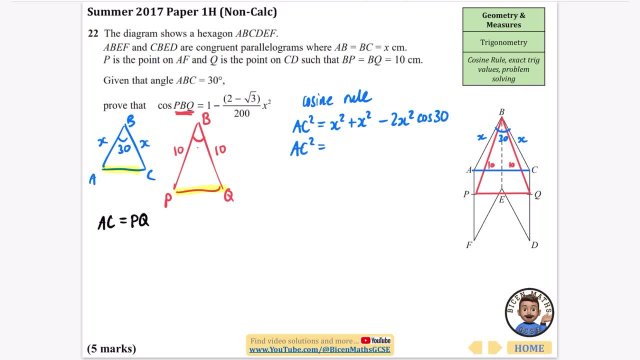 cos of the angle, which is 30. So AC squared is 2X squared minus 2X squared multiplied by cos of 30. This is the exact value you need to know. Cos 30 is root 3 over 2.. So I'm just going to write that. 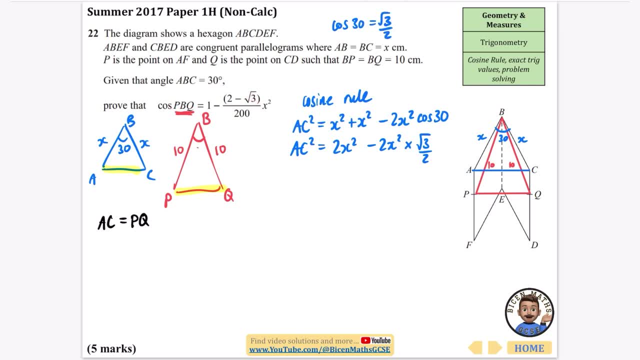 down that cos 30 is root 3 over 2 and there's a bit of a clue because of that root 3 that we've got there. So my final bit of simplifying is that it is 2X squared, 2X squared multiplied by root 3. 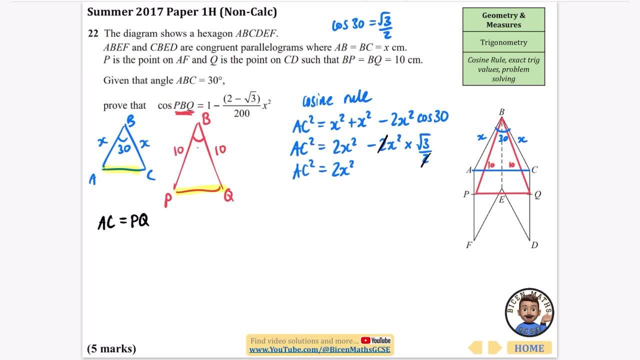 over 2.. Well, those twos that we have here in the triangle are going to be equal to 2X squared, So I'm just going to write that down here. They're going to cancel, so that what we get left with is 2X squared minus root, 3X squared minus root, 3X squared. Okay, now I'm going to do the cosine. 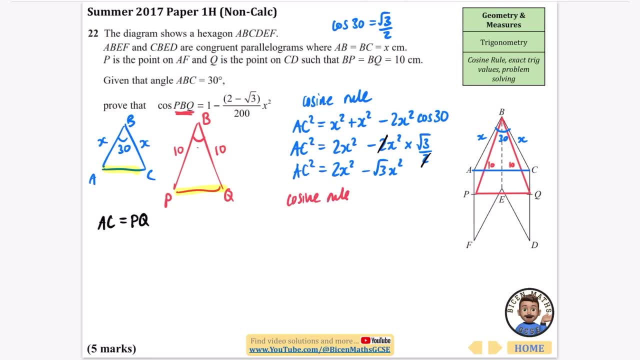 rule for the red triangle. So I'm going to do the cosine rule for the red triangle. It's in a very similar pattern. that PQ squared is going to be my 10 squared plus 10 squared, That's the B squared plus C squared minus 2 times B times C. So 2 times this times this, That's 2 times 10 times 10.. 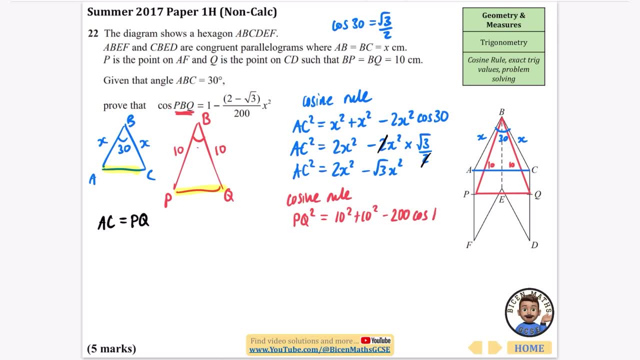 That's 200 cos of the angle which we're talking about, which is PBQ. Remember, that's the thing we're actually trying to find here. So we get that PQ squared is equal to 100 plus 100. That's 200 minus 200 cos of PBQ. Now I know that AC is equal to PQ, which also means that AC squared must be. 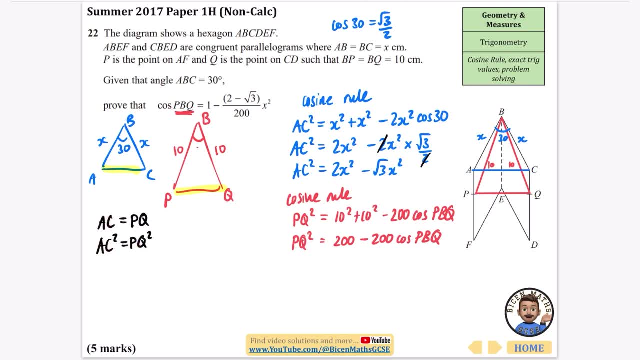 equal to PQ squared, because if it's the same length, it'll be the same when it gets squared. So this means I can take this thing and this thing and make them equal to each other because that when they're squared they are equal to each other. So my last part of working is that 2X. 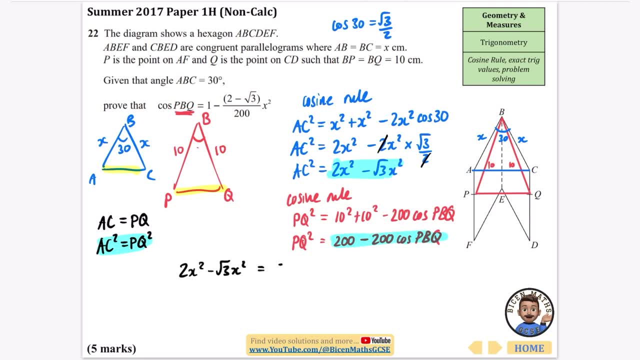 squared minus root. 3X squared must be equal to 200 minus 200 cos of PBQ. Now I like to do a bit of factorising. I noticed that I could take a factor out of X squared here so that I get my 2. 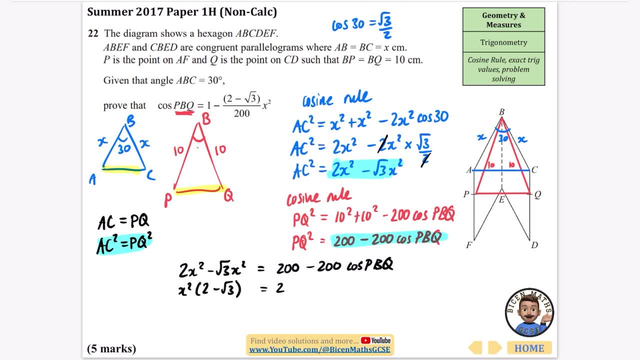 minus root 3.. And if I also take out a factor, I'm probably not going to take out the factor of this bit. What I might do is, instead, I'm going to put this 200 cos of PBQ onto this side, So I get 200 cos of PBQ. 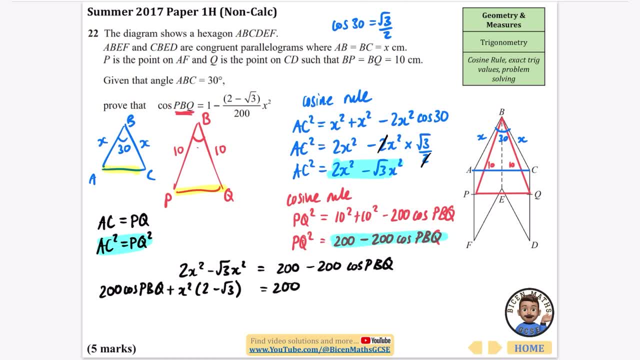 plus this equals 200.. So my last step is to subtract this to the other side. Well, it's my penultimate step, actually. So I get that 200 cos of PBQ is 200 minus X, squared 2 minus root 3.. All that's left is to divide everything by 200 and make sure that it looks. 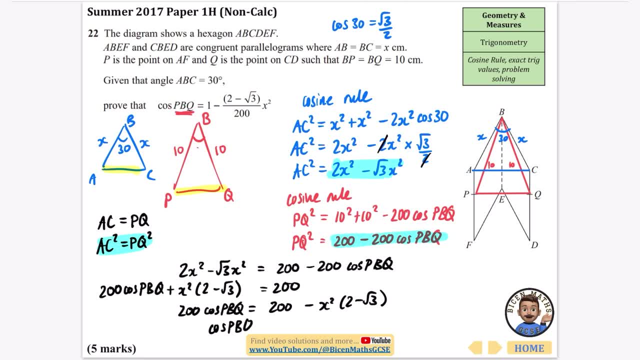 like this. So my cos of PBQ is 200 divided by 200 is 1, and then this divided by 200 is my 2 root, 3 divided by 200, and I'm just going to put the X squared at the end, just like where theirs was. 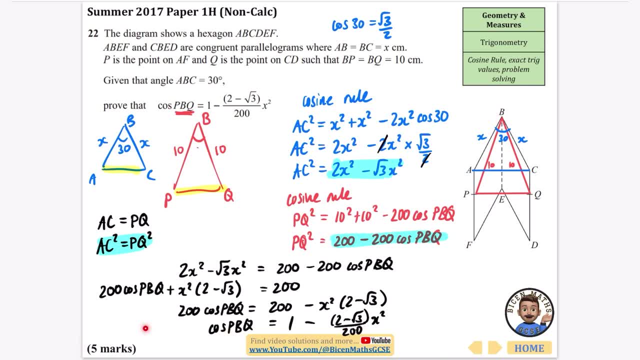 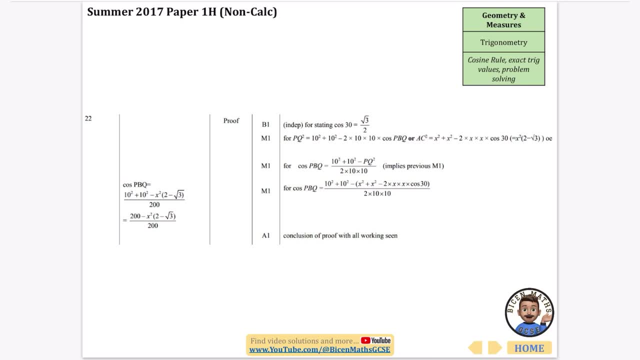 And so I've shown that this is the thing that is true. A very difficult question. It's right, one of the last questions in the paper and it is worth five marks, So you could try and read it all through here, but I hope my version of it's going to be a little. 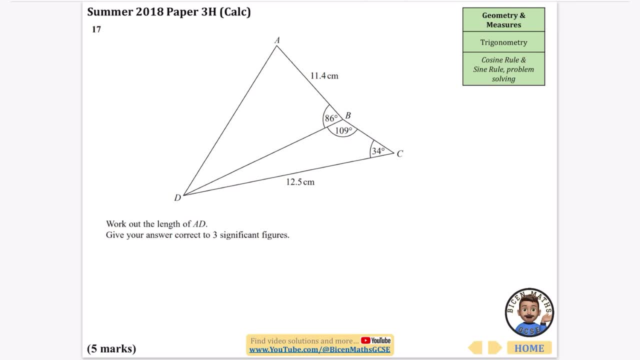 bit more helpful for you. Okay, now a slightly easier one after that very tough question. So it says: here we want to work out the length of AD. So this is the thing that I'm aiming to try and find out about, and I'm going to give my answer to three significant figures. Well, as usual, 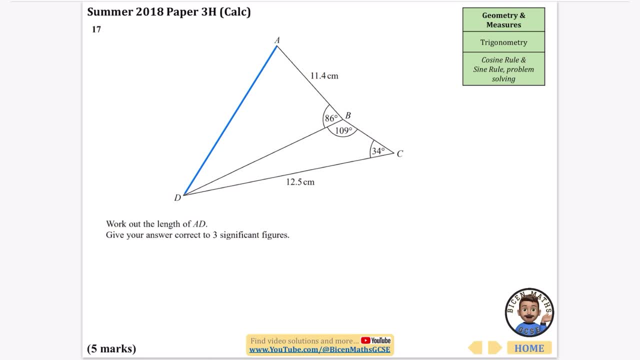 let's just do some work on this triangle. I think actually I'm going to end up finding that one, So I might change that one to a different colour. I'm going to start off trying to find out the length of BD, Because if I find out the length of BD I've probably got enough information for that second. 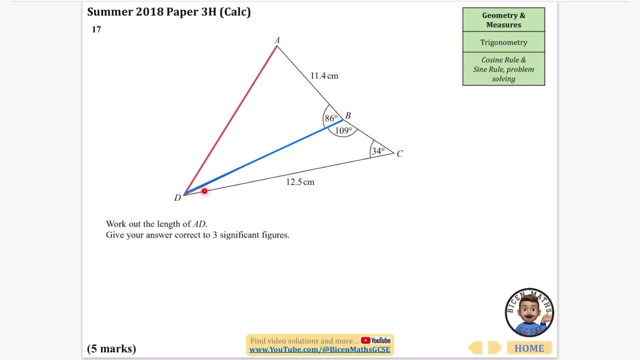 triangle, So I'm going to concentrate on this one to begin with. Okay, I'm going to look at this triangle here Now. you'll notice I have got an angle and the one that is opposite it, and I have got an angle and the one that is opposite it. So I'm going to start off by saying that. BD. 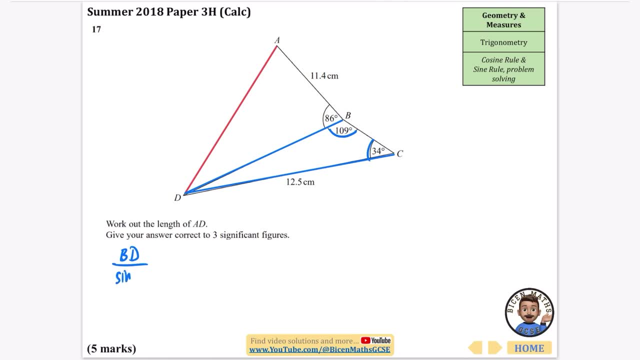 this is the sine rule. BD over the sine of 34 is equal to the other length, which is 12.5.. Over the sine of 109.. So that will tell me what BD is. It's going to be 12.9, 12.5, sorry. 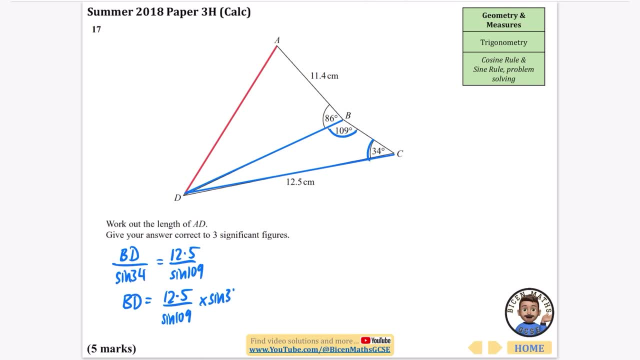 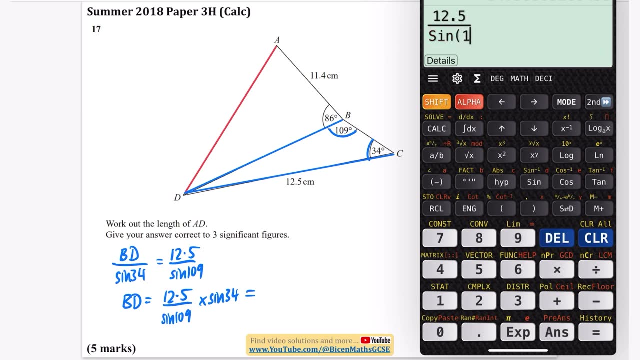 over the sine of 109, multiplied by the sine of 34.. And I'm going to get that all onto my calculator straight away. So we have 12.5 divided by the sine of 109.. That is going to multiply by the sine of. 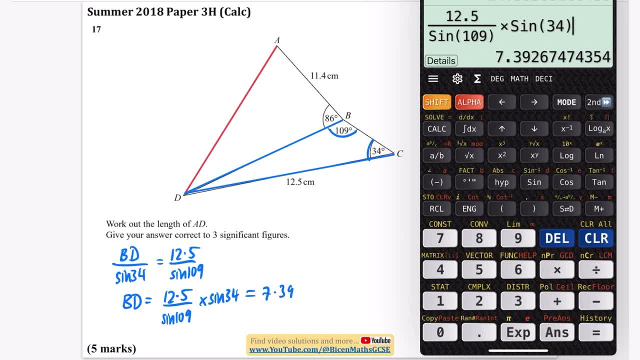 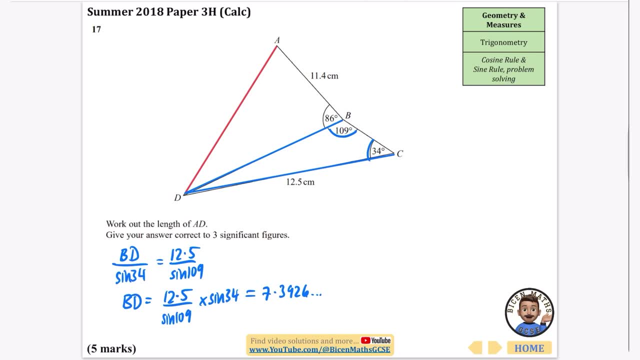 34. And that is 7.3926. blah, blah, blah, And I'm going to put the dot dot dot to show it keeps going And I'm just going to keep it stored On my calculator there. Okay, Now that I know that this length here is 7.3926.. I can have a 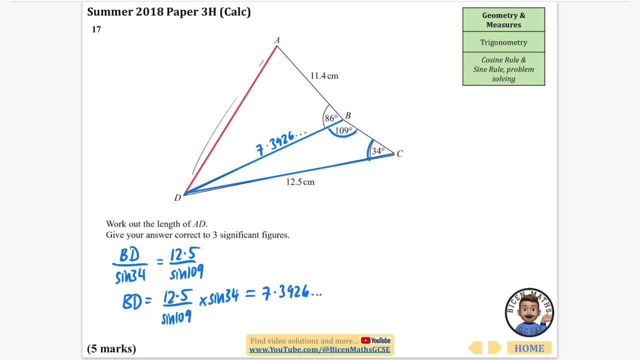 think about what's going on in this sort of red section that we've got. We're trying to find out the length of AD that we have And I think we might be able to do the cosine rule for this, because we've now got in this triangle. I've got a side that I know about. I've got another side. 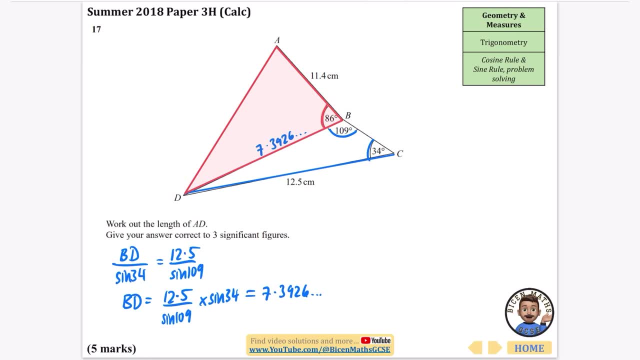 that I know about And I've got the angle that goes between them, which means that I can do the cosine rule in red. So I'm now going to do the cosine rule in red. So I'm now going to do the cosine rule. And remember our cosine rule is: A squared equals B squared plus C squared minus 2BC. 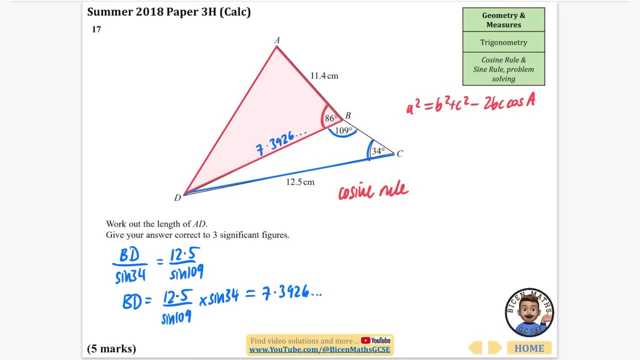 cos A, And the crucial thing is that this and this are opposite each other. So this one is opposite the angle We are good to go, Which means that AD squared is equal to the other two sides squared. So that is going to be my 11.4 squared plus my 7.39, blah, blah, blah squared minus 2 times 11.4.. 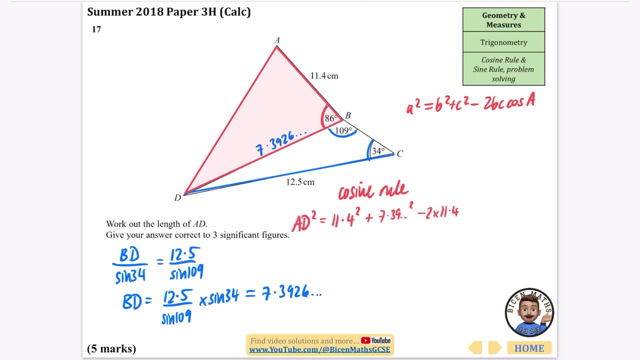 This is going to have to move across. So I've got some more space: 2 times 11.4 times my 7.39 blah, blah blah multiplied by the cos of 86.. So I'm actually going to find out what AD is by typing this: 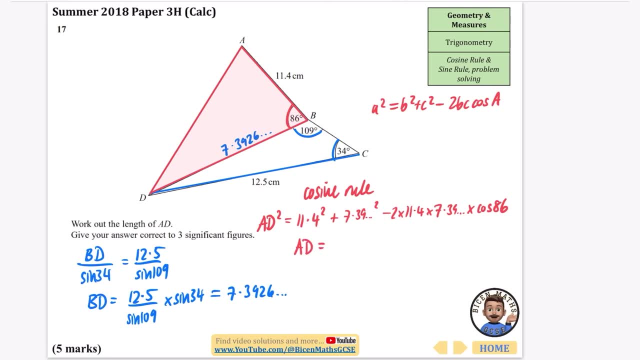 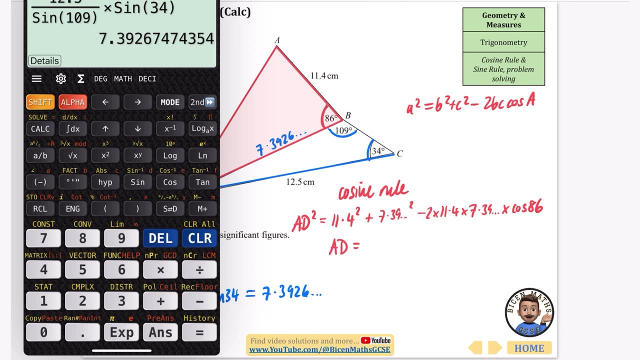 into my calculator with the square root sign in it. But I'm just going to save myself a little bit of time doing that Now. remember, I've already got that horrible seven point number stored in the calculator, So I can just do the square root of 11.4 squared plus the answer squared minus 2. 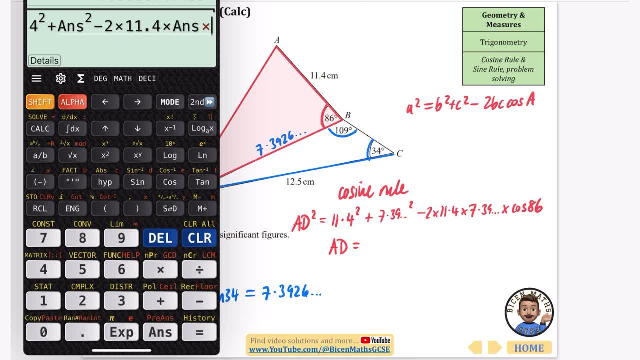 times, 11.4 times, by the answer times, by the cos of the angle, which is 86.. And we get the answer to three significant figures, That is 13.1.. 13.1 centimetres. Let's double check to see that we've. 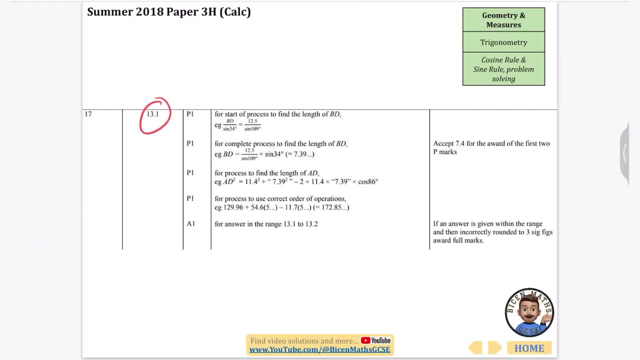 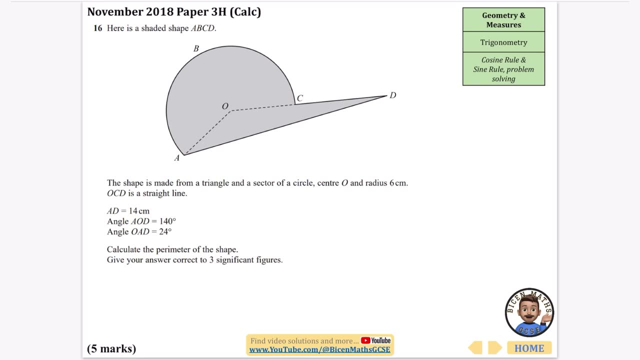 got this one right, please. So we do have 13.1.. And you'll see in the process that we've got like the sine rule followed by the cosine rule down here. Okay, this one is weird because we're blending it together with some sort of sector of a circle. So we just want to. 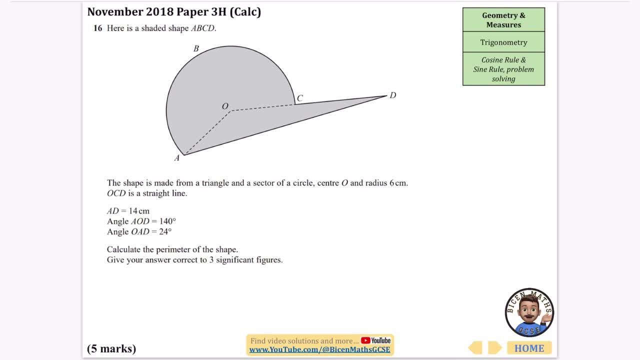 read through and make sure we add everything into the diagram, because this one they haven't labelled a tonne of stuff. The shape is made from a triangle and a sector of a circle, centre O and radius six. Okay, so that immediately is telling me that this is six and between O and C. 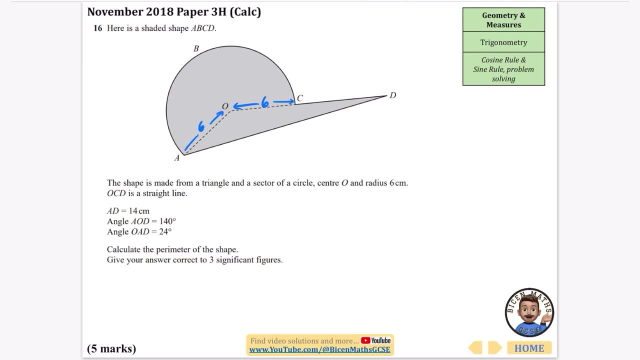 I'm just going to make that clear that it's just between O and C, that is equal to six as well. It then says that AD is 14 centimetres angle AOD, so the one in the middle of those three letters. 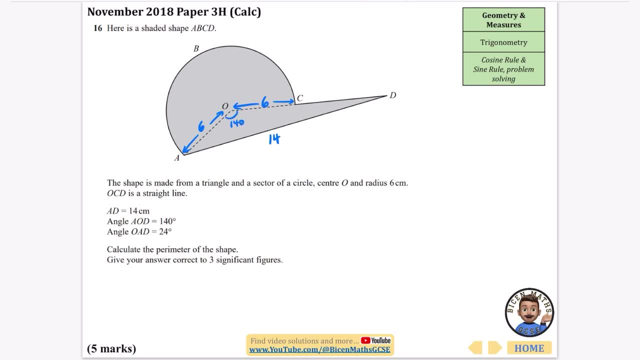 that is 140.. And then angle: OAD. OAD is 24 degrees, So this one here is 24 degrees. that we've got. Now, if I need to, I know I can find this one because of angles in a triangle. So I tell you what I might do that. 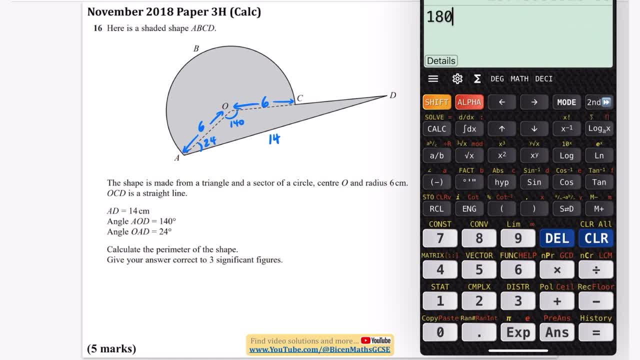 just because I think that's the kind of thing that they like to do in these sorts of questions. So I'll do 180 minus 140 minus 24.. So that one is 16. And if I use it, great. And if I don't use it. 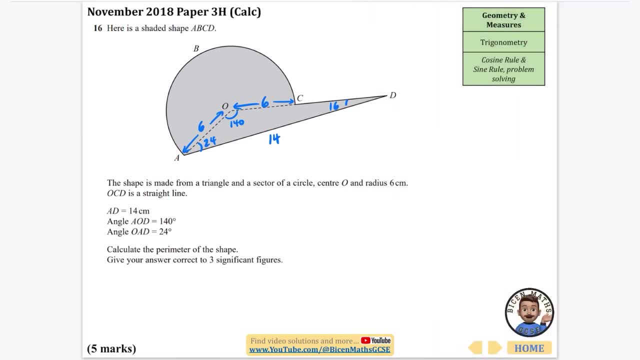 it's not an issue at all. Let's just get rid of that little bit at the bottom. Okay, so now we're actually going to see what we're want to do in this question. They want us to find the perimeter of this shape. We're going to try and. 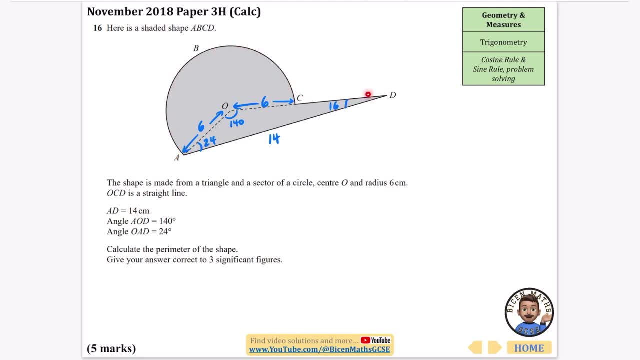 see what the distance is from here to here, and then between C and D and then along the bottom. So I think what we're going to do to start off with, I think we're going to find out the perimeter just of this particular shape that we've got here. So we're going to discuss the sector of the circle. 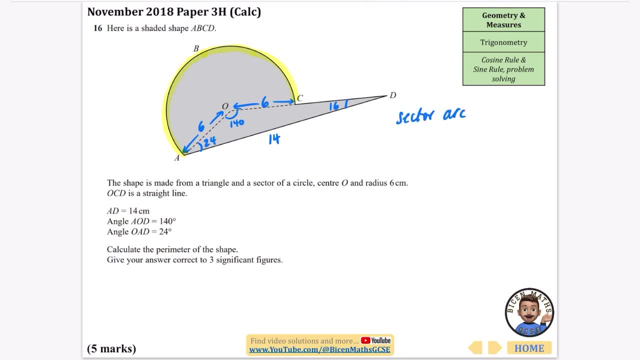 the sector arc, And the arc just means this part that we've got here. So let's highlight that so you know we're talking about the same thing. Well, I guess that the angle that we have- because that's 140, this is going to be 360 minus 140, which is 220. 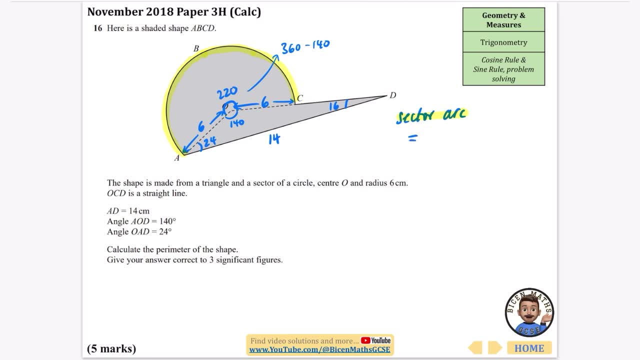 So the sector arc is going to be equal to the fraction of that whole circle. So that's 220 out of 360 multiplied by the circumference. Now remember, the circumference of a circle is pi multiplied by the diameter. So it's going to be pi multiplied by the diameter of the circle. 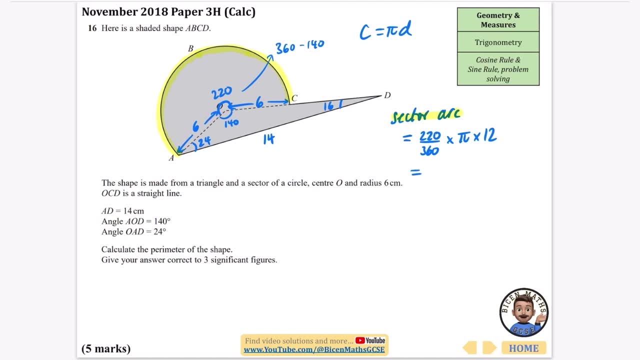 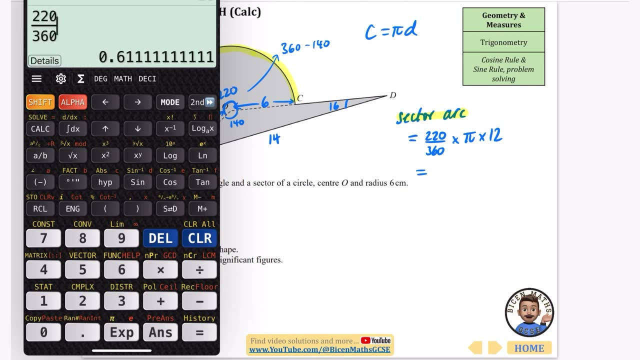 which is 12, because the radius is 6.. So let's find out what that's going to be. So we're going to do 220 out of 360.. We're going to multiply that by pi, and we're going to multiply that by 12.. And so that we get this is 23.038. blah, blah, blah. 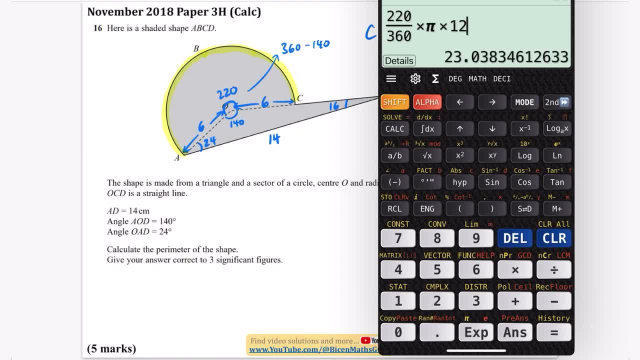 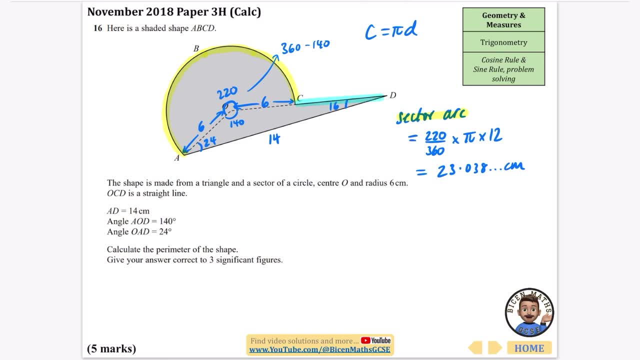 centimetres, And we're going to come back to that one later on. Now we're going to try and figure out how long this part is. Now, in order to do that part, I think we're going to need to find out the whole of this shape that we've got. 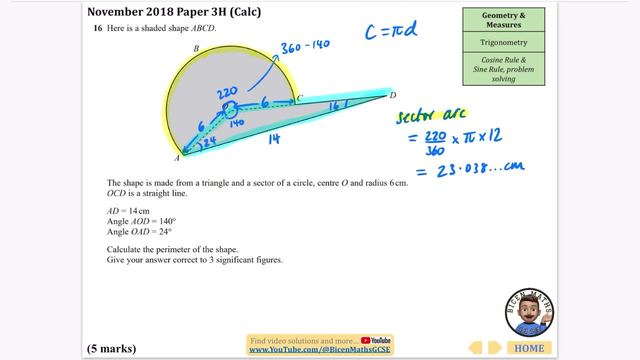 Not the whole of this shape, But the whole of that length. We're going to try and find out the length between O and D. I might actually draw out that little triangle because I think it might help us visualize what is going on. So this is a 6. OD is the thing I'm going to look for, And this is 14.. And I know all. 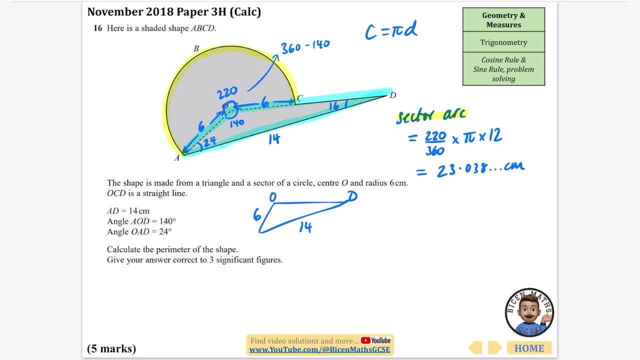 of the angles that are in here, So I'm actually going to use the ones that are opposite the sides that I know. So opposite the 6 is the 16. And opposite the 14 is the 140.. Oh, actually that's. 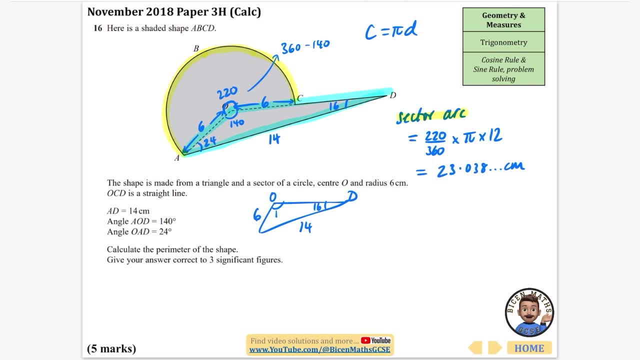 not the ones I want to use. I don't want to. I want to find out the length of of this side here. So actually I want to know this angle. Those are the ones I'm going to use. I actually don't even need to use these two. I can do these two. So let me correct what I've. 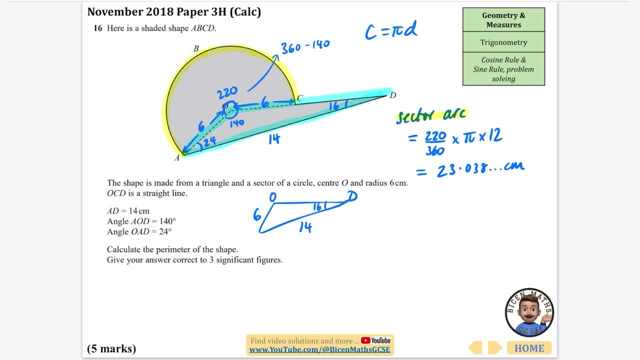 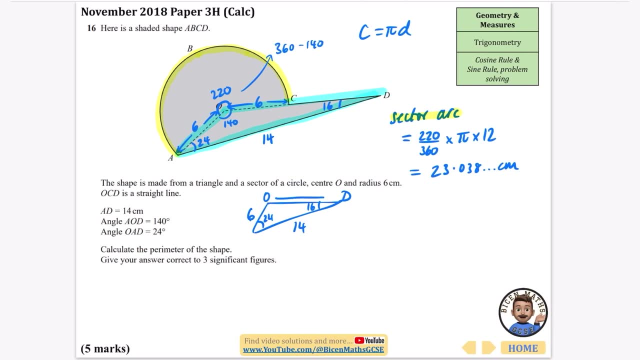 got on my diagram. We're going to use the 6 and the 16. And I know this angle is 24.. And this is the one that I'm looking for. So I'm going to say, as that is the side that I'm looking for, 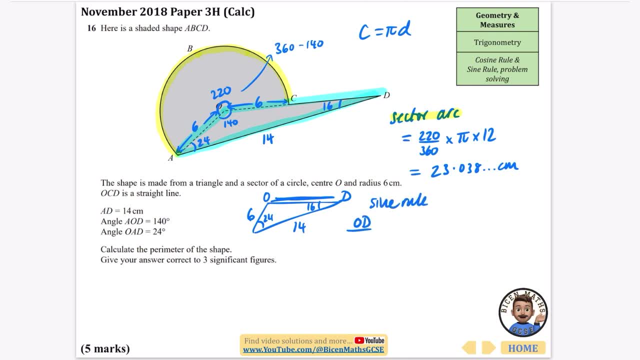 using my sine rule, that OD divided by the sine of 24 is going to be equal to another pair. Now I could do the 14 and the 140, or I could do the 6 over sine 16. It's going to literally give us: 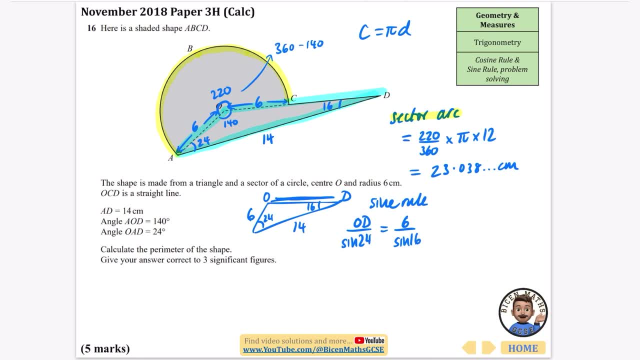 the exact same answer. So if I do 6 over sine 16, this will tell me that OD is 6 over sine 16 multiplied by sine 24.. Let's see what this gives us. So that is going to be 6 over sine 16. 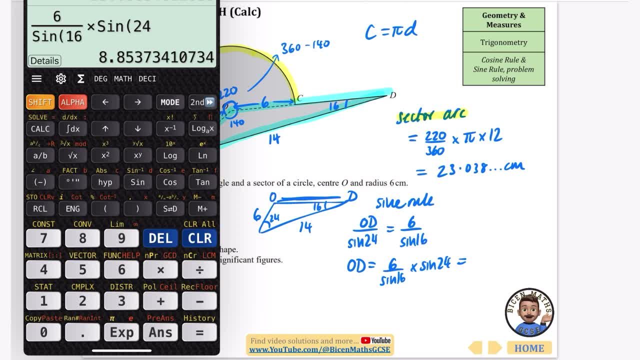 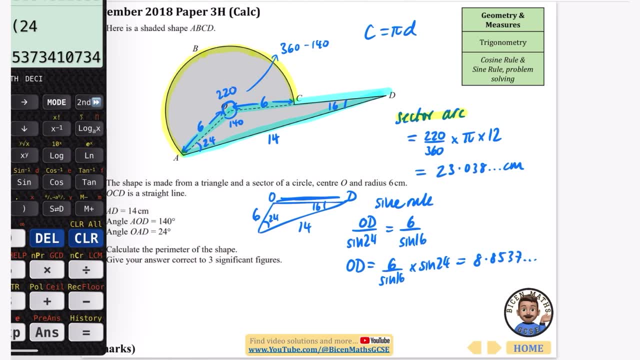 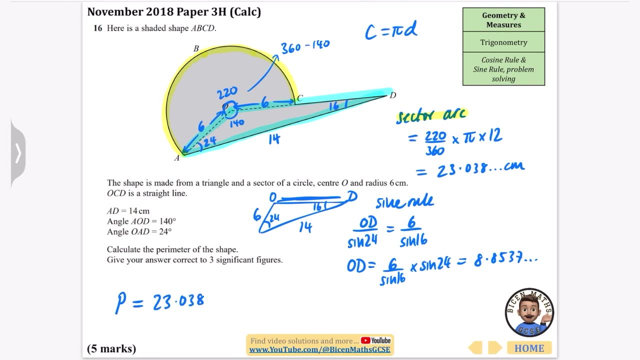 multiplied by the sine of 24.. And we get that OD is equal to 8.853, 7 blah, blah, blah like this. So the perimeter of the shape is going to be equal to the yellow part that we've got, which is my 23.038.. Then I'm going to add on the 14 that I've got along the bottom. 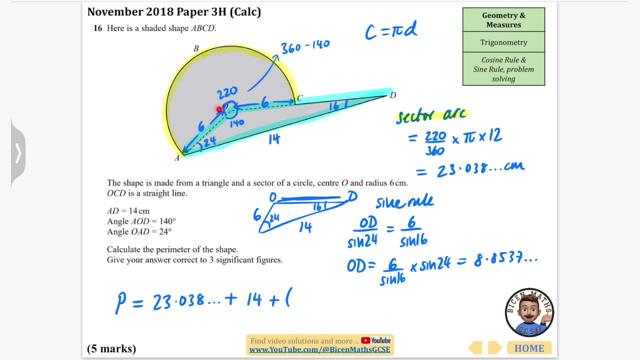 And then I'm going to add on: well, this part that we've got here is 8.8537.. And I only want this CD length. This CD length is going to be this one minus 6.. So it is going to be my 8.8537 minus 6.. 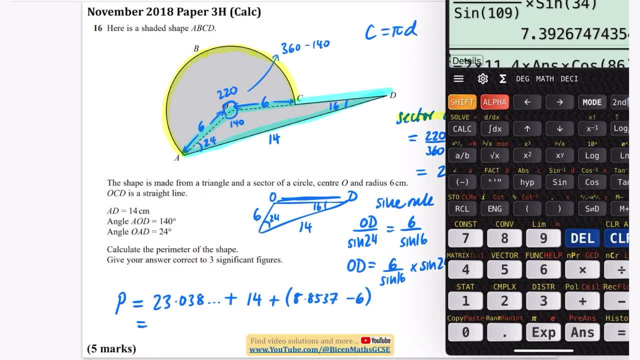 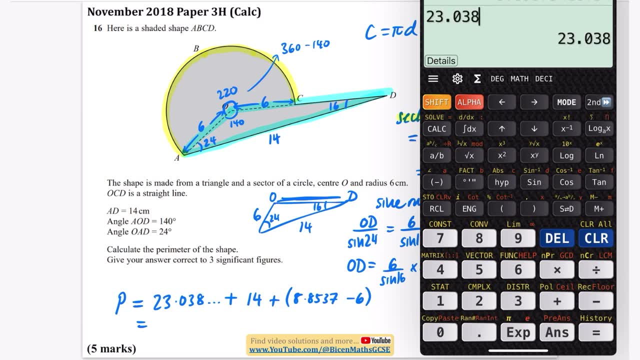 If I put that all together it should give us the perimeter. So sliding the calculator back over to this side. Remember, I've got that 8.857 stored as the calculator, So I'm going to type in 23.038 plus 14 plus the one that's on the calculator, that 8.8537 minus the 6.. Oh, didn't mean to do. 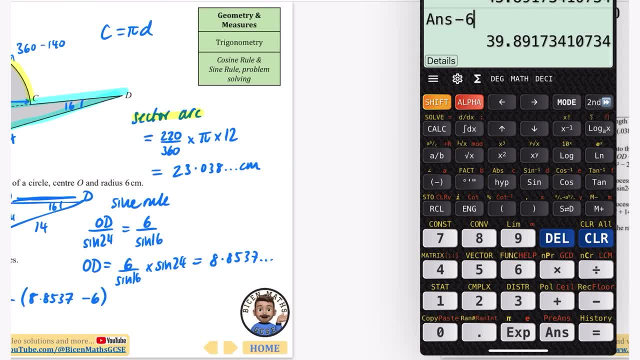 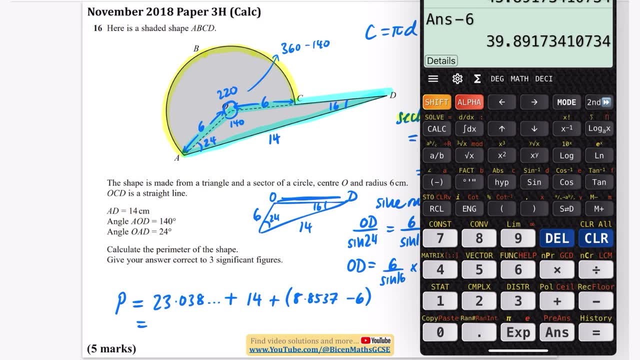 that bit. So if I just press minus 6, it should work. I'm worried I've done something funny when I typed it. No, I haven't, I have done that all correctly on my calculator. I just pressed equals twice And we get that the perimeter is equal to 8.8537 minus 6.. So if I just press minus 6, it should. 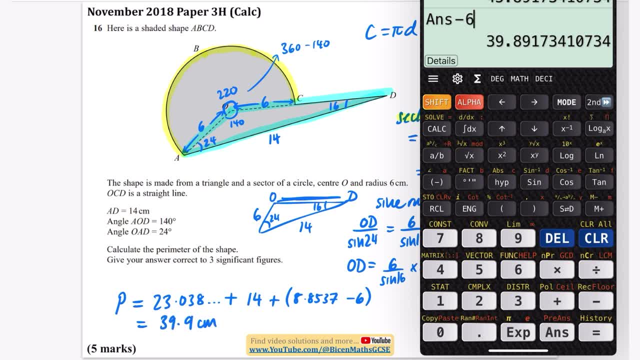 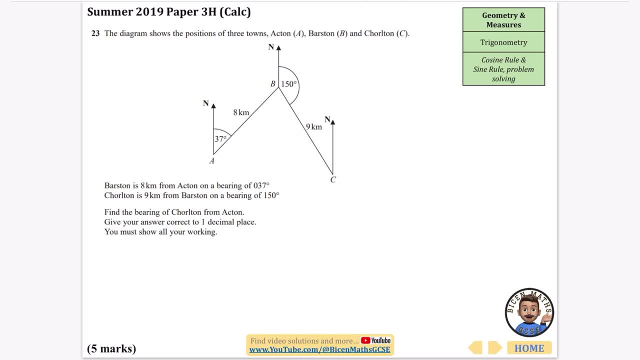 work. So we get that the perimeter is 39.9 centimetres, which I can just see on the next page, is the right answer that we have here. Okay, we have now got a bearings kind of question, but it is basically just a trig one. If it's question 23,, it's likely to be sine and cosine. 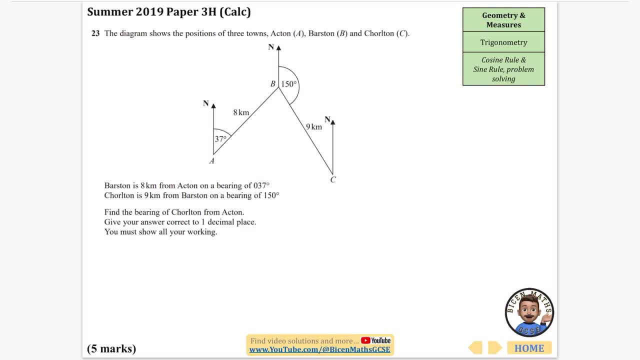 rule. It's so late in the exam paper. So it says that Barston is 8 kilometres from Acton on a bearing of 37.. Chorlton is 9 kilometres from Barston on a bearing of 150.. Find the bearing. 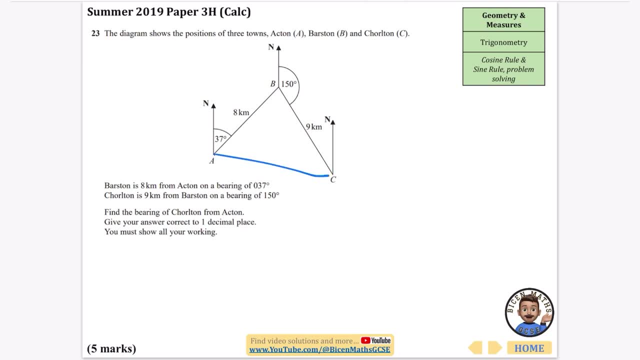 of Chorlton from Acton. So I'm going to press minus 6.. So if I just press minus 6, it should going to start off by just joining these two lines together, and I'm going to try and find out what. 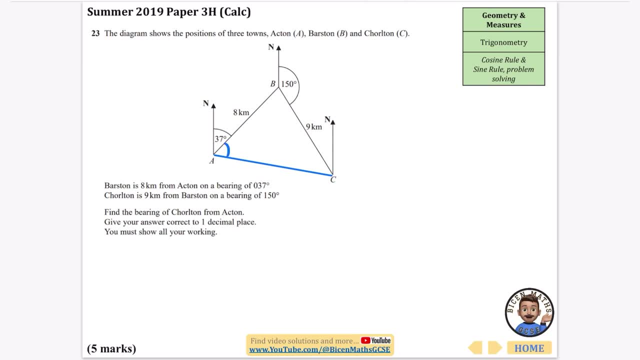 that whole bearing there is. in other words, I kind of need to find out what this angle is, because then I can put them together to find that out. and it wants us to give up to one decimal place. well, look what I've got. I have got the side, and I have got the side, and I think what I'm going to 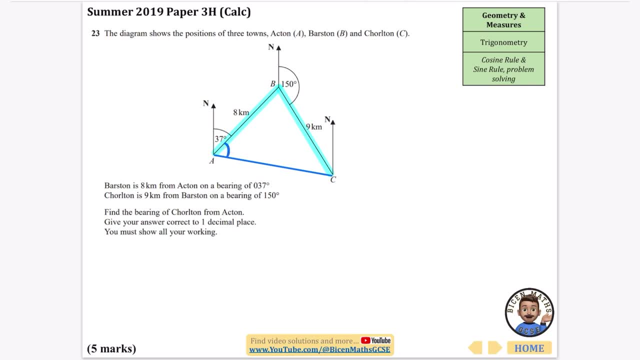 need to do. if I'm going to try and find out what this angle is, I think what I could try and do is find out this side. then I will find out something to do with an angle. sorry, let me say this again: I'm going to try and find out this angle which will allow me to find out this side, and then I 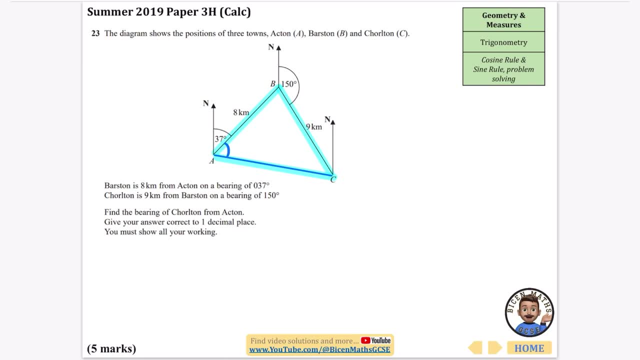 think I've got enough to do the sign rule with all of this stuff that we've got going on now. this is why this question is really difficult, in my opinion. I think I can find out what this angle is using the properties of bearings. first of all, if this is a vertical line and this is 150. 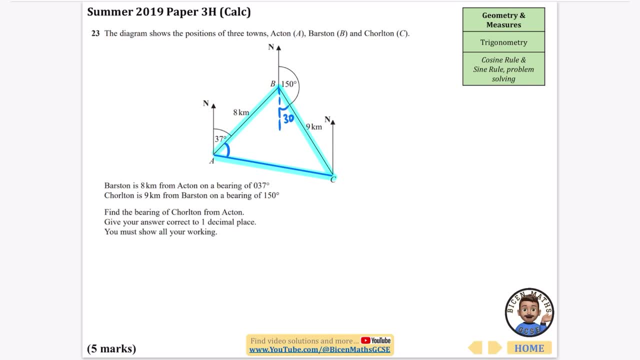 then this is 30. similarly, if these are parallel- which they are because they are parallel- then I can find out what this angle is, and I can find out what this angle is because they're the north line. if that's 37, that must be 37, because they are alternate. 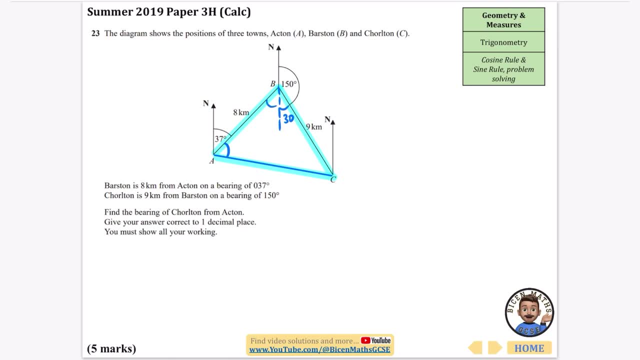 angles, which sometimes people call z angles, but they are alternate angles, which means that is 37. so if I redraw this triangle that I've got- and it's going to be a very sketchy version of it- I have my a, my c. this angle at the top is 67, this is 8 and this is 9. so I'm going to figure out what. 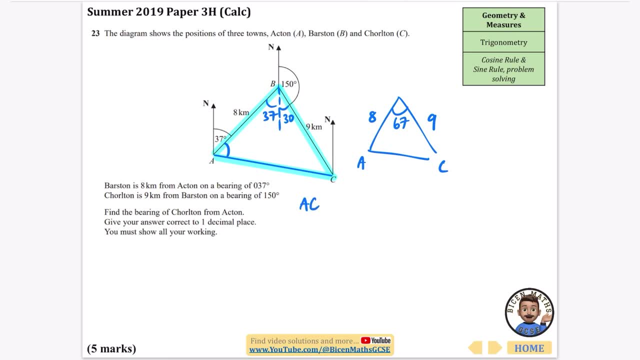 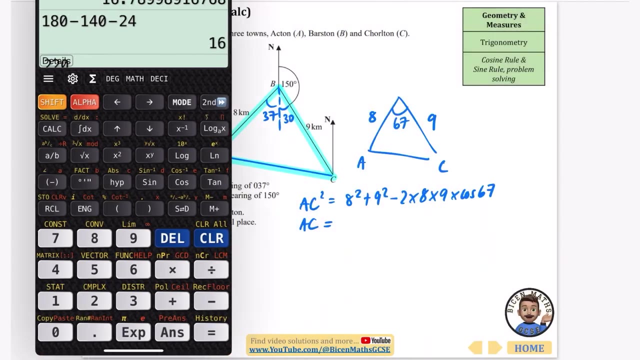 the length ac is. now ac is going to: ac squared using the cosine rule is 8 squared plus 9 squared minus 2 times 8 times 9 times the cos of 67. so I can figure out what ac is by typing that in, but obviously with the square root sign. that's going to go above it as well. so I'm going to do. 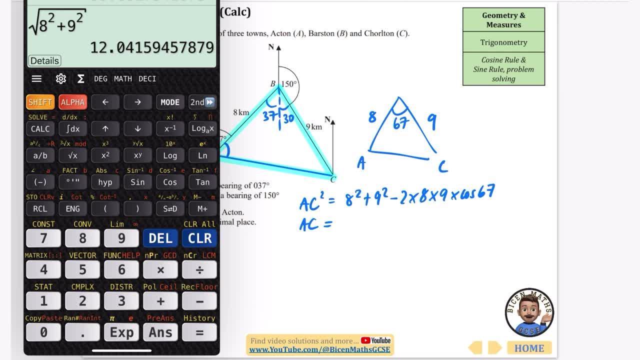 the square root of my 8 squared plus 9 squared always starts off a bit like Pythagoras: minus 2 times 8, times 9 times the cos of 67, and we get that ac is 9.4199. I'll tell you what. when I use 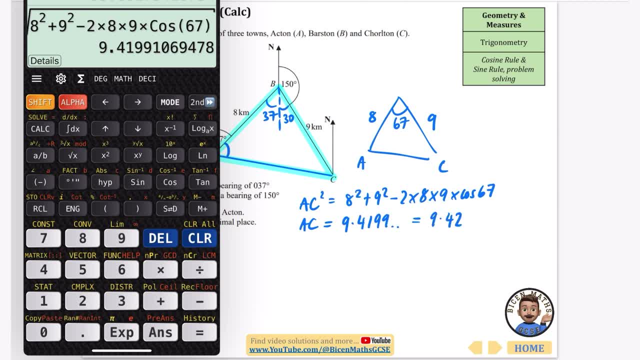 it. in my calculations it's actually so close to 9.4199. so I'm going to do the square root of my 8 squared is 9.42. I'm just going to use it as 9.42 kilometers. so if I now go back to here, this is 9.42 kilometers. 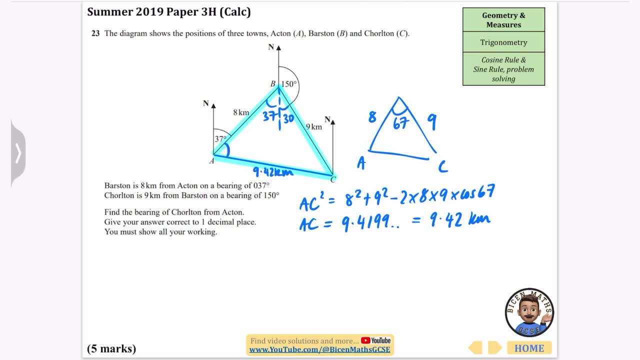 remember. this is the angle I'm trying to find out. so I actually think I've got enough information to do this and, you know, if it's a five mark question, you're probably going to be doing the sine rule and the cosine rule once each. maybe maybe some other bits as well. so I know that this. 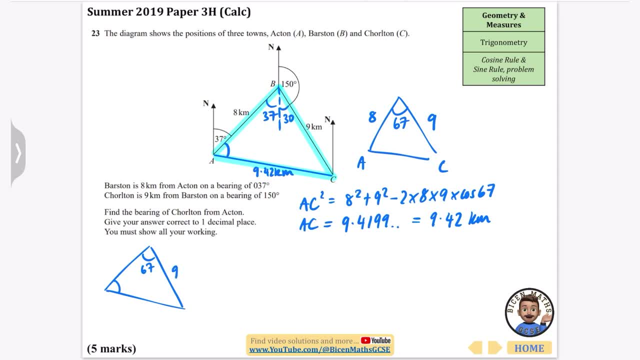 is 67. this is the angle I'm trying to find out- that one has opposite a 9 and the one that I have opposite here is my 9.42. so if I call this angle x for a second, I'm going to say that the sine of x over 9 is equal to the. 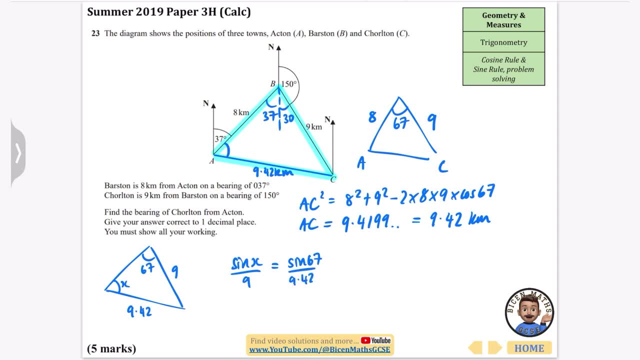 sine of 67 over my 9.42. so this means that sine x is going to be sine 67 over 9.42 multiplied by 9, and then I'm going to find out what x is by doing the inverse sine of that in just a second. but 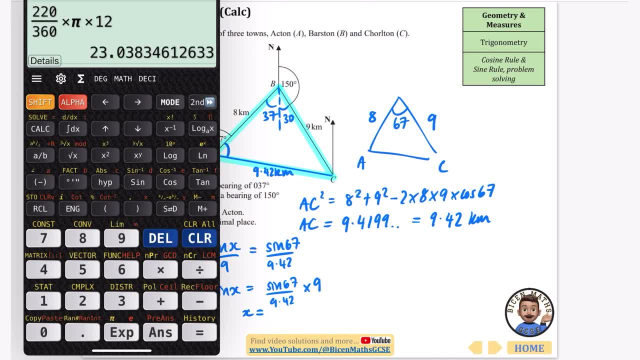 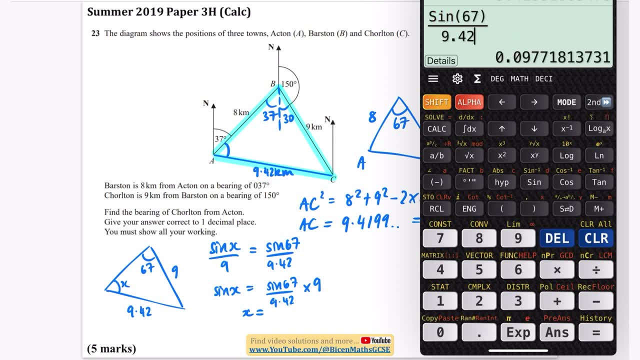 let's get some of that on my calculator. so, typing this in, we get that the sine of x is equal to the sine of 67 over my 9.42. so if I call this angle x for a second, I'm going to the sine of 67 over 9.42 multiplied by 9. is this answer that we get? so let me just write down what. 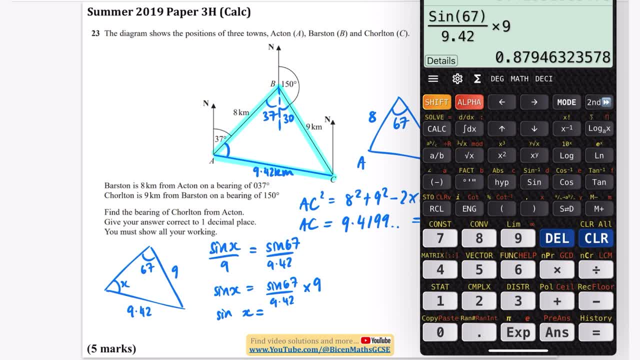 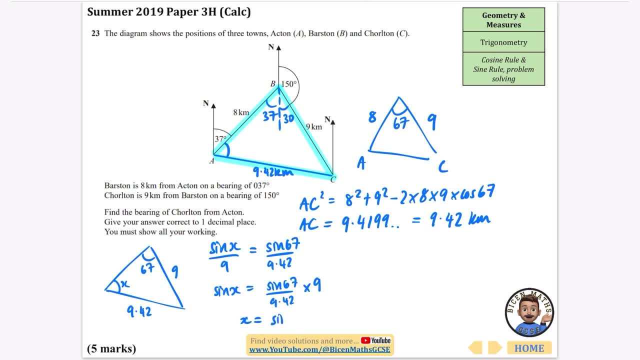 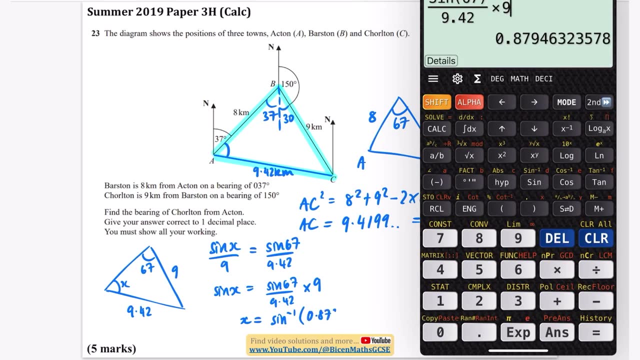 x is equal to. actually, I'm not going to do that. I'm going to write down that we can do the inverse sine of that. so x is going to be the inverse sine of what we've just worked out to find out what the angle is. and that is. where's that all gone on my calculator? 0.8794. now I'm just going to keep it. 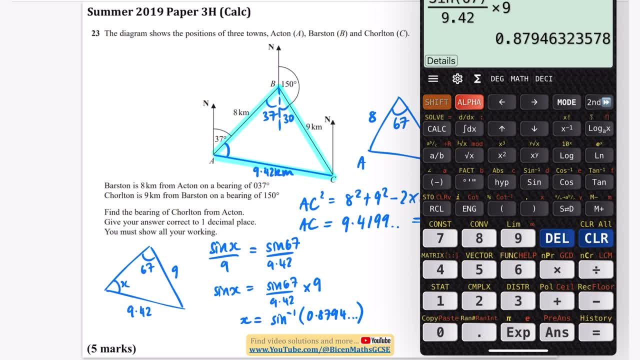 stored in my calculator, which is why I don't need to worry about writing down all of the numbers. so I'm going to do the inverse sine of the answer that my calculator had and that is going to give me that x is 61.6 degrees, and that's to one decimal place. therefore, my final step is to say: 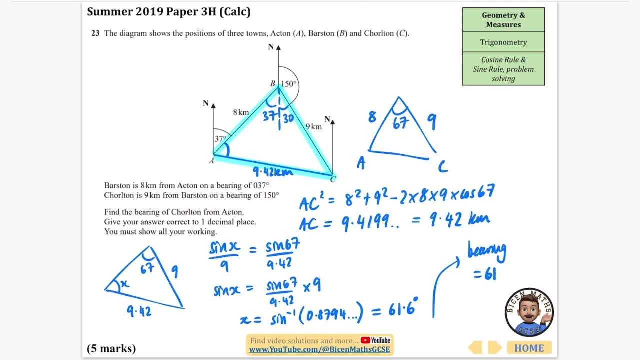 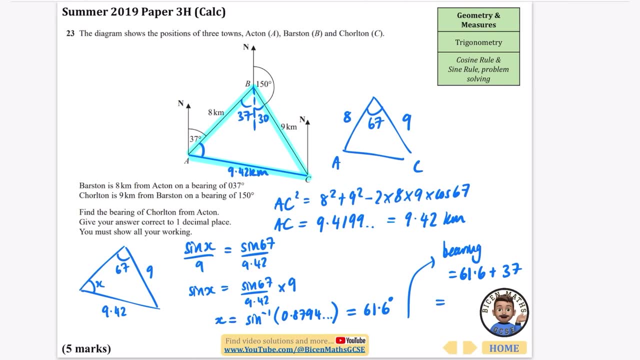 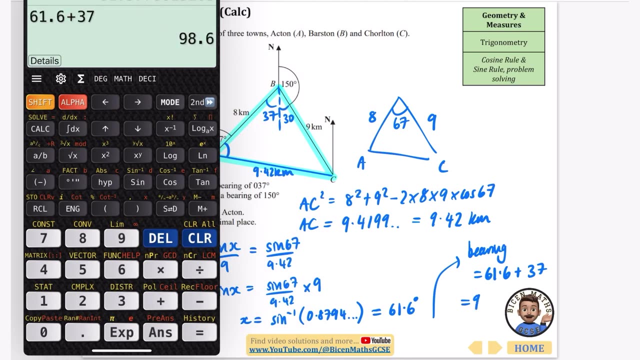 what the bearing is equal to. so the bearing is going to be 61.6- and it was okay to round it there- plus that 37, and so my final answer for this is 61.6 plus 37. I probably don't need a calculator, but I'm going to do my 61.6 plus 37, and I get that it is 98.6 degrees, but because it 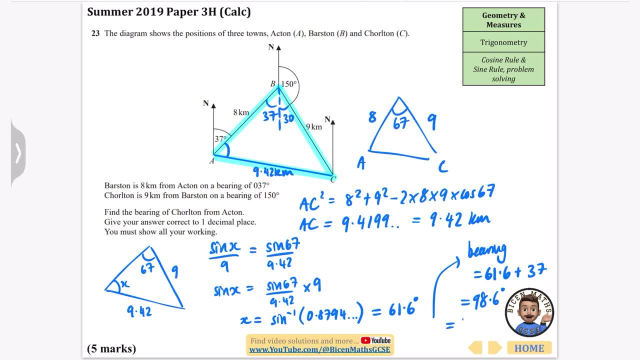 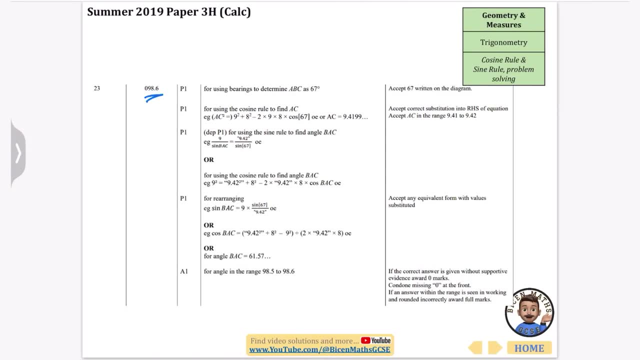 wants it as a bearing. we should actually put at the beginning a zero, so it is 098.6 degrees. let's double check that we've got this one. there is the 0.986 and we've got the correct part. now they actually would accept it like this. I don't think it says condone a missing zero at the front. 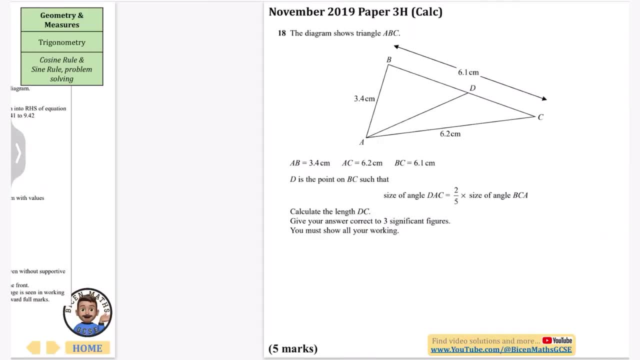 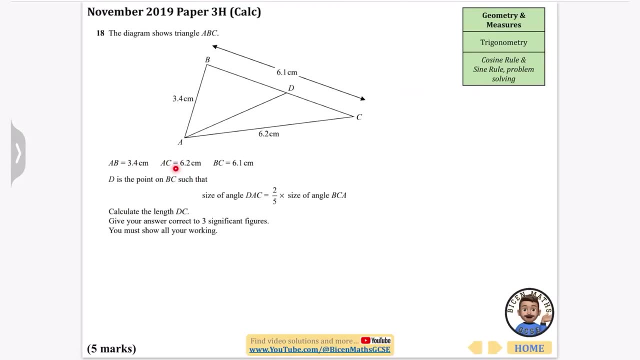 so if you didn't have that missing zero at the front, that would be perfectly okay in this question. okay, we are nearly there. I think we've got two questions left. well done for sticking with it so far. so all of this information is basically on the diagram, apart from this part. it says the size of 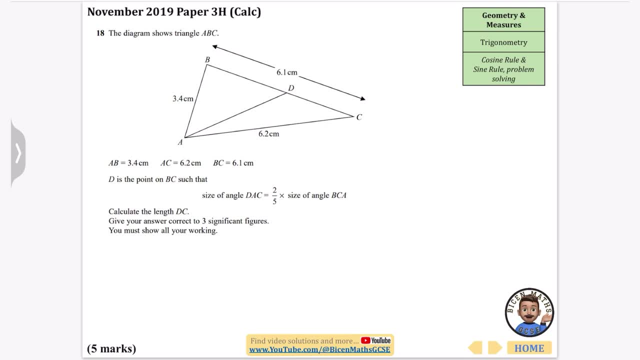 angle dac is two-fifths of the size of angle bca, so I'm going to go and call this one 5x. and then if I'm going to say I want two-fifths of that, well, a fifth of that is x, which is why I picked 5x. 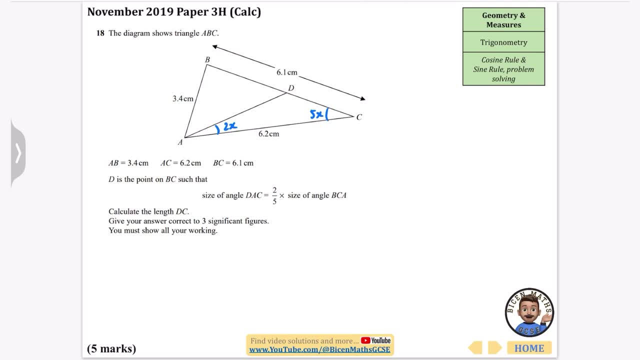 and if you times that by two you get 2x and it wants us to calculate the angle dac, the length of dc that we've got here. we're going to try and calculate that length. well, I think we've probably got some information with this large triangle and we know that one of the sides 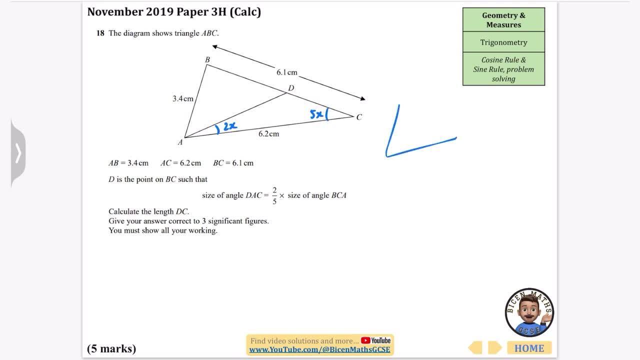 is 5x. so if I look at the large one, this is going to be the way I'm going to find out what the size of x is. so I have a 5x, a 6.1, a 3.4 and a 6.2 and I'm going to do the cosine rule. so the cosine rule. 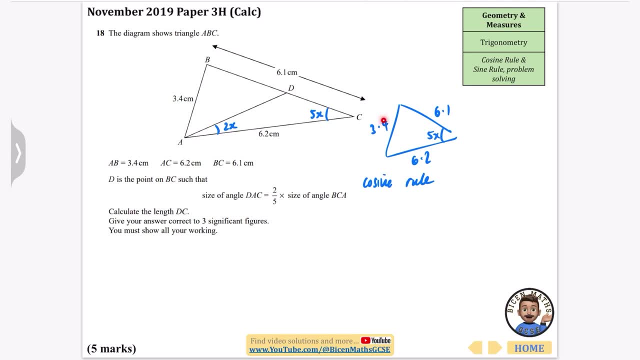 some people remember this rearranged, but I actually just don't. so I'm going to say that it's: this one squared equals this one squared. so I'm going to do the cosine rule and I'm going to do this one squared plus this one squared minus. two times this times, this times, the cos of this. 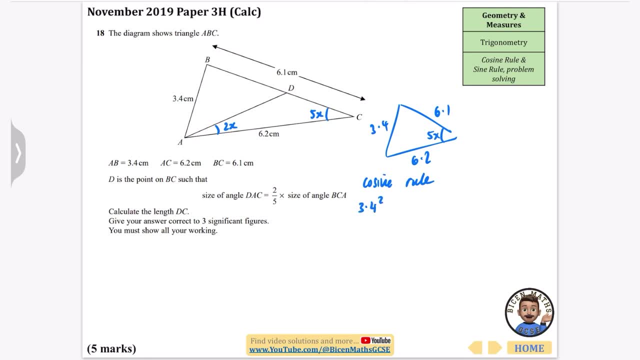 so pretty intense. so it is: 3.4 squared equals 6.1 squared plus 6.2 squared, minus two times 6.1, times 6.2, multiplied by. let's see if I can just slide this over, so I've got a bit more space. 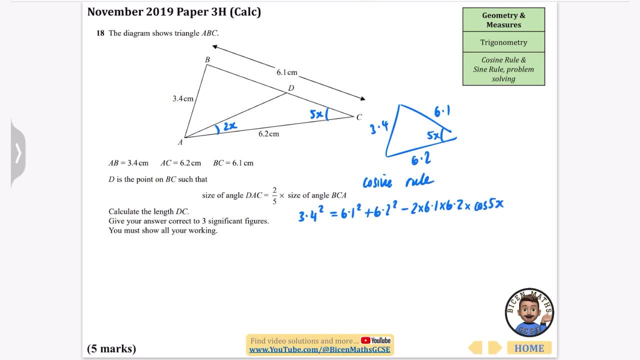 multiplied by the cos of 5x. now some people know how this rearranges. if you want to do this as a rearranging, you can do this minus this minus this. you can do this minus this minus this minus this, divided by this whole thing. so that is going to be my 3.4 squared minus 6.1 squared minus 6.2. 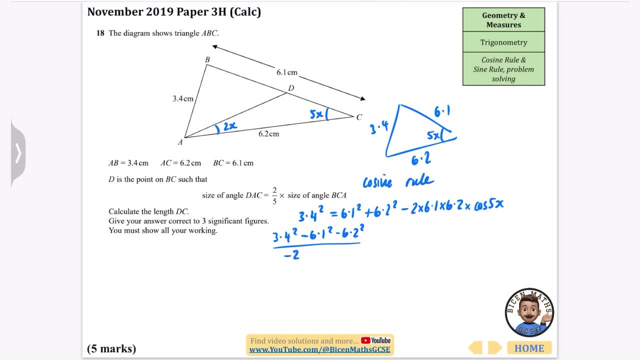 squared all divided by minus two, because there'll still be a negative two at the beginning, it's going to be minus two times 6.1. times 6.2, that is the cos of 5x. so I'm going to use that to find. 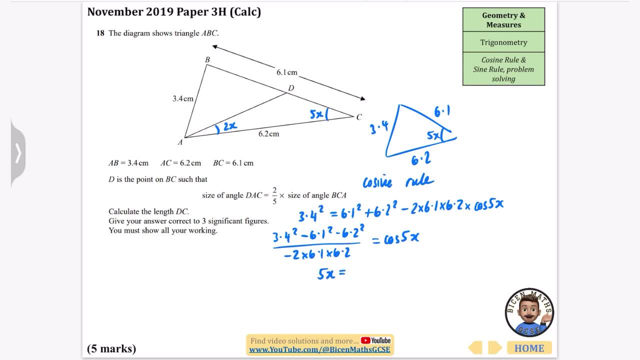 out what 5x is equal to by saying that 5x is therefore going to be the inverse cos of that whole thing: 3.4 squared minus 6.1 squared minus 6.2 squared minus 6.2 squared minus 6.2 squared. 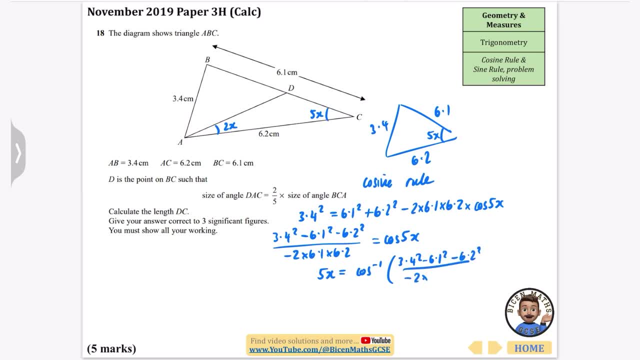 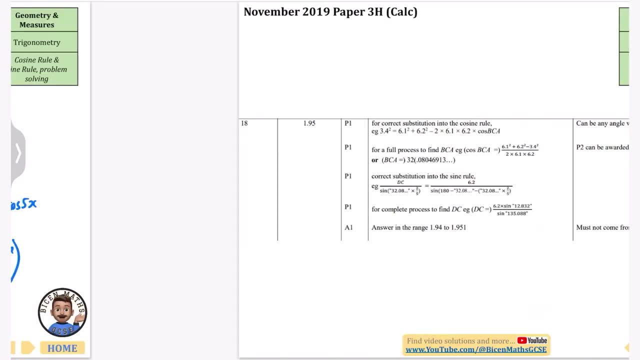 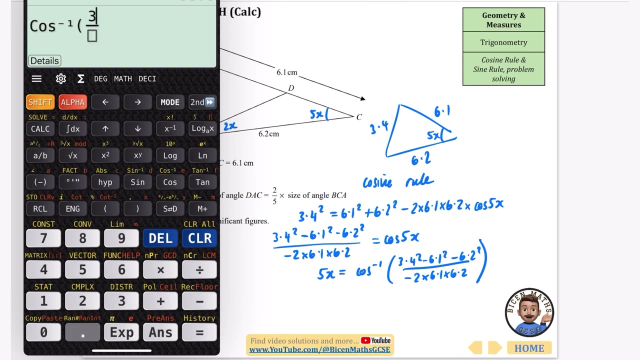 all over minus 2 times 6.1, times 6.2. okay, that will then tell me what X is. then we can keep going on this pretty insane question. to be honest, oh yeah, of course the calculator is on the other side, so I'm going to do the inverse. cos of get this as a fraction, we're going to do our 3.4 squared minus. 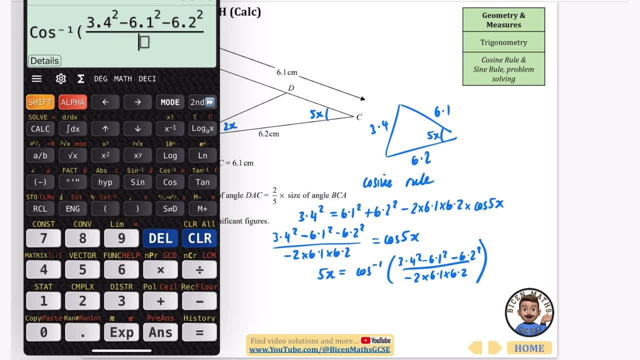 6.1 squared minus 6.2, squared all over negative 2 multiplied by 6.1, multiplied by 6.2, and that is telling me what 5x is equal to, and that's going to be the inverse cos of 5x squared minus 6.2 squared. 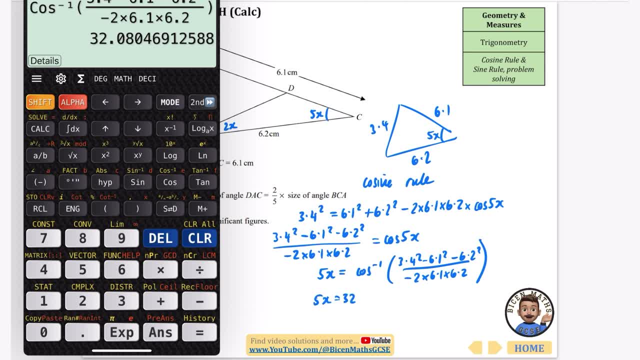 so 5x is 32.08 degrees. so I can find out what X is equal to by dividing it by 5. and if I divide that by 5, I get that X is 6.416 degrees. so I'm going to need some more space. I'm going to need 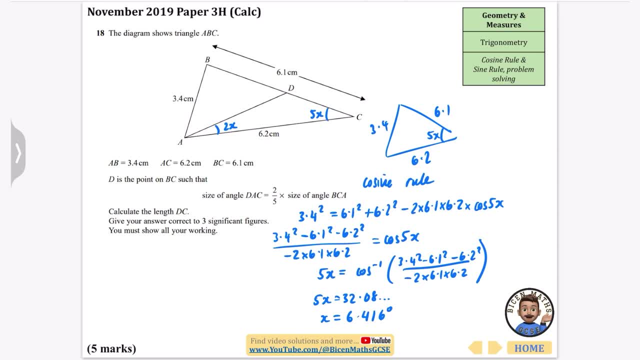 to come over to this part of the page. so I now want to find out what the length of DC is. well, I think I might need to find out what these angles are. so this is 2x. I'm going to say that 2x is. 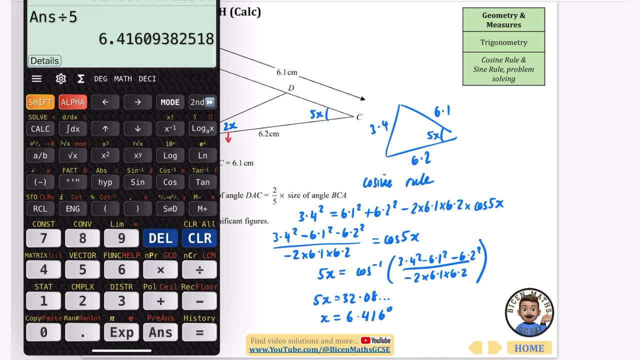 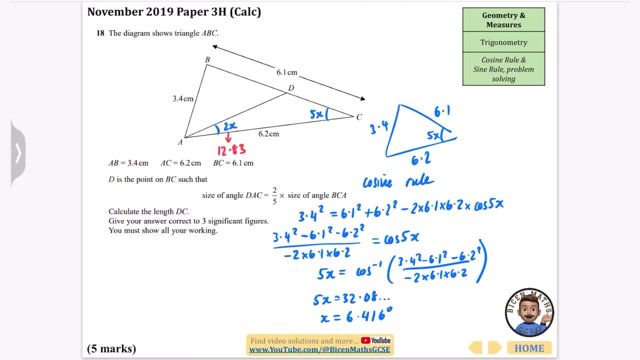 double that one that I've got on my calculator. so let's multiply that by 2, that is 12.83. so this is 12.83, the 5x I can find out as well. I think I've actually got the 5x- it was down here as 32.08- and then I can find out what this other angle at the 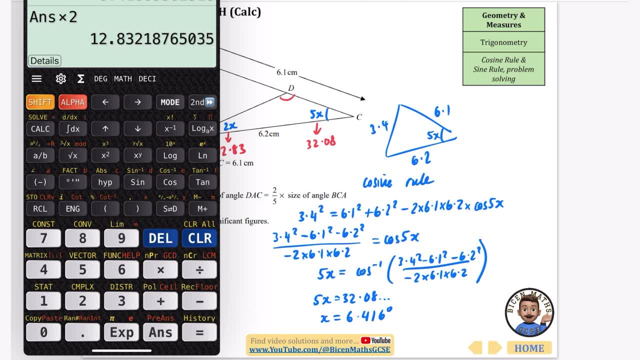 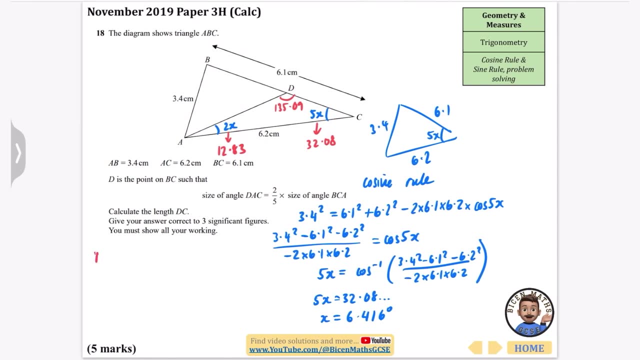 top is as well, by doing 180 minus that. so that is going to be 180 minus the 12.83 minus 32.08, so the one at the top is 135.09. and now I'm going to find out what the length of DC is. so DC divided by the sine of this, which is: 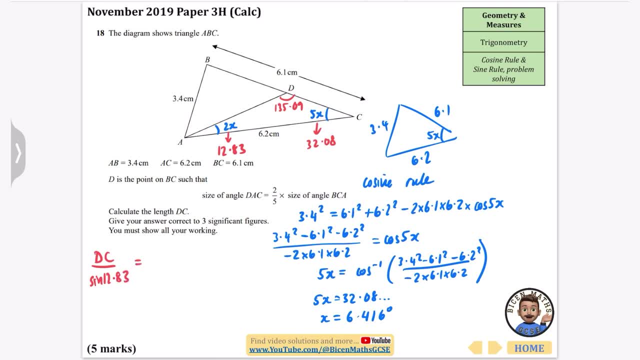 the sine of 12.83 is equal to- I can say this length because I know this one- divided by the sine of that. so that is going to be 6.2 divided by the sine of 135.09, and I'm actually just going. 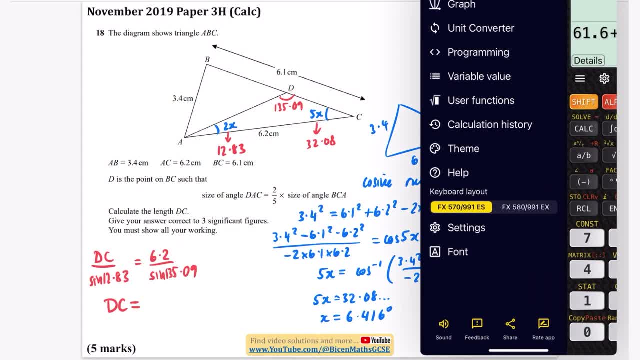 to put this all in my calculator. to save us a bit of time, I'm going to do the division and I'll multiply it by the sine of 12.83. so that is going to be 6.2 divided by the sine of 135.09. 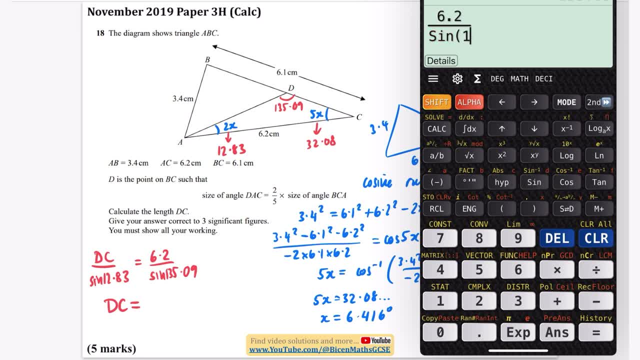 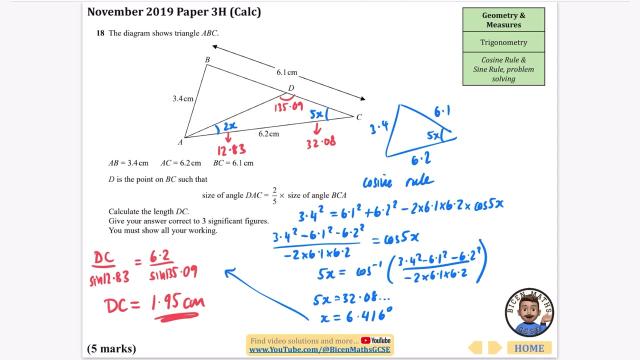 so that is 6.2 over the sine of 135.09, multiplied by the sine of 12.83, and we get that DC is to three significant figures, 1.95 centimeters. so I'm just going to quickly say on here from my working. it then kind of comes up to: 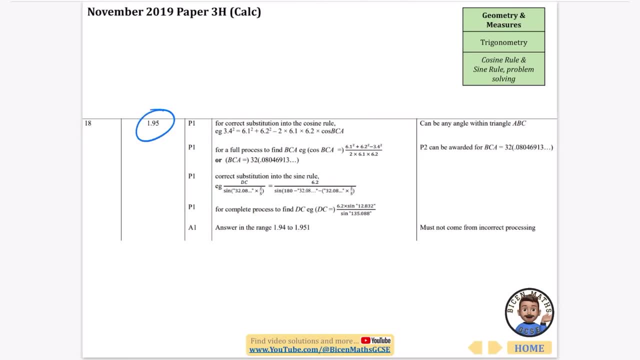 that place. let's save, see if we've got this one right. there is the 1.95. what a relief. so I'm just going to quickly say on here from my working: it then kind of comes up to that place because I kind of do these questions a bit on the fly, so it's very good for me to see when I've 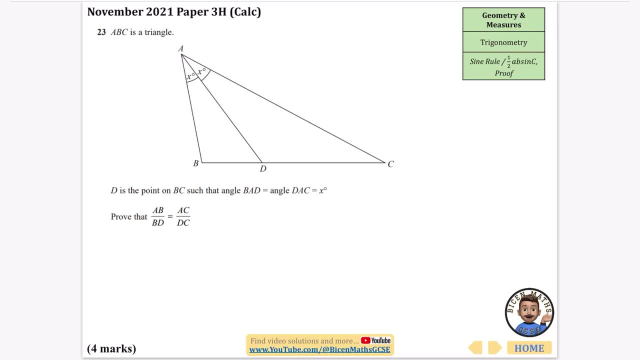 got them right, okay. last one in this section and it is tough. it's the last question. if it's 23, I should think we have ABC as a triangle. D is the point on BC, so that, should the angle BAD and angle DAC are both equal to X, prove that we've got these kind of things here. this looks a bit like it's. 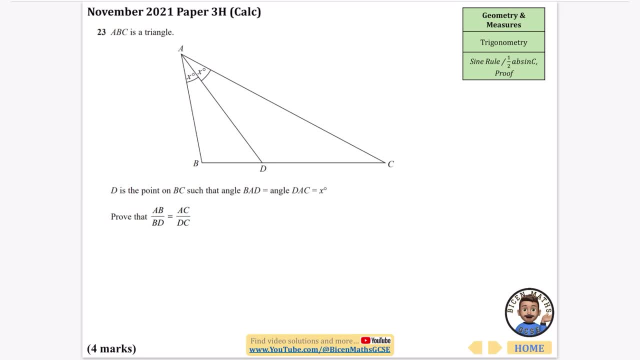 come from some kind of ratio. now what I'm going to do- this is probably not the way that my people might see this. this is just the way that I would see this one. I'm going to try and compare the area of these triangles and I'm going to try and compare the area of these triangles and I'm going to try. 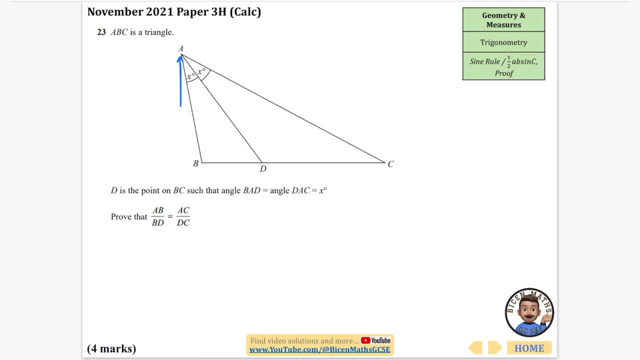 and compare the area of these triangles, and I'm going to try and compare the area of these triangles in two different ways. one of the ways I'm going to do it is the very simple way of just saying: I've got the height of the triangles, so both of them have got a height of H. you can see that they. 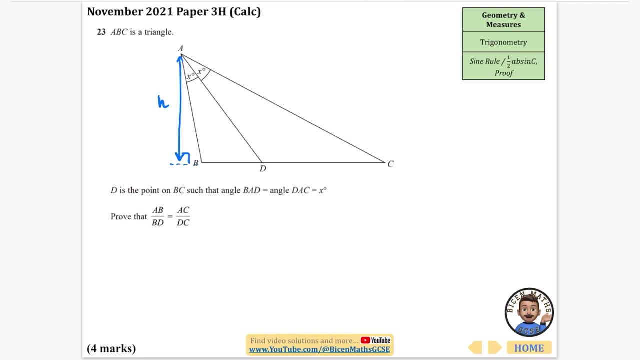 both have a height of H, and when I say a height, I mean it's like the perpendicular distance. so I can say that the area of this triangle number one, and then I'll do triangle number two. so for triangle number one I could say that the area of- yeah, let's just do this- the area of triangle one. 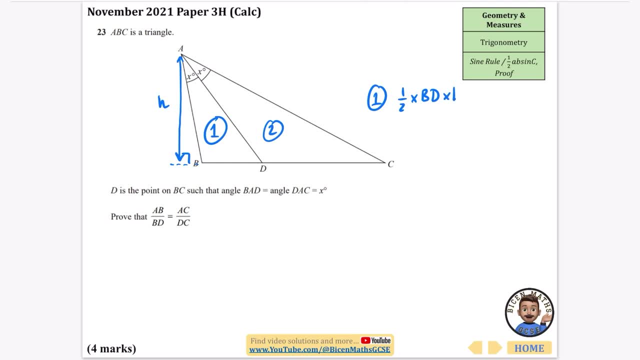 is a half multiplied by the base multiplied by the height. the area of triangle two is a half multiplied by the base multiplied by the height. but I could also work out the area of triangle one in a different way. I could use my half a B sine C, which would be a half multiplied by a. 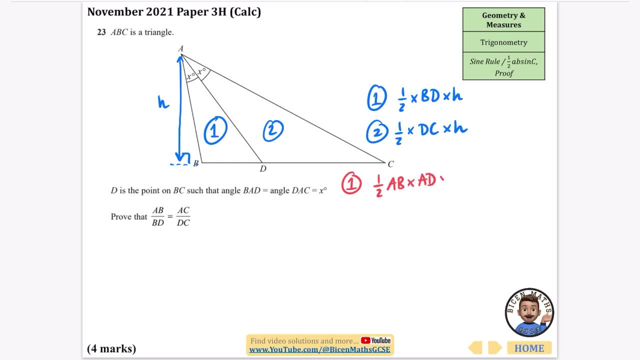 B multiplied by a, D multiplied by the sine of the angle between them. and for triangle two, I could do the same thing. I could say that it's a half x, the two the this side and this side. So that is going to be my AD multiplied by AC multiplied by the sine. 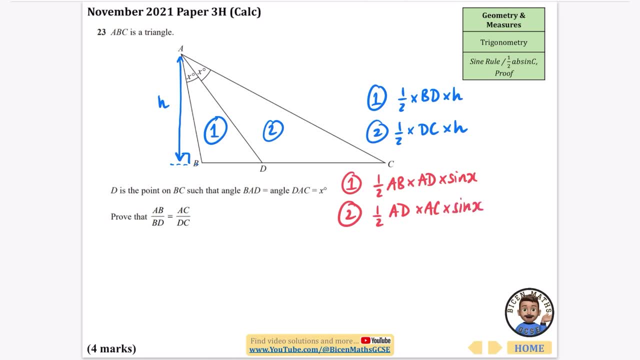 of the angle between them. Now, I should know something about these things. I should be able to say that the area of one triangle divided by the other should be the same as this one divided by this one Kind of doesn't matter which way round that I do it, If I'm going to do triangle. 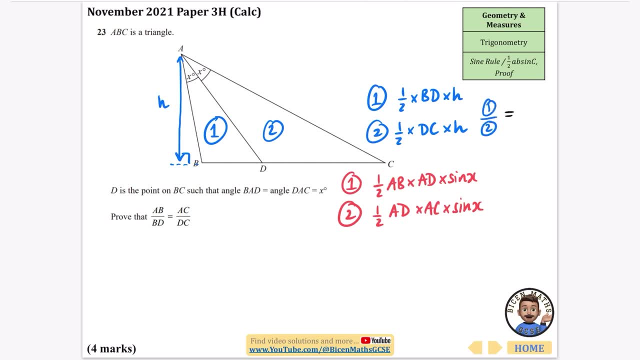 one divided by triangle two in blue. that should be equivalent to doing triangle one divided by triangle two in red, because we're talking about the same triangles that we've got here. In other words, this one as a proportion of this one is the same as this one as a proportion of. 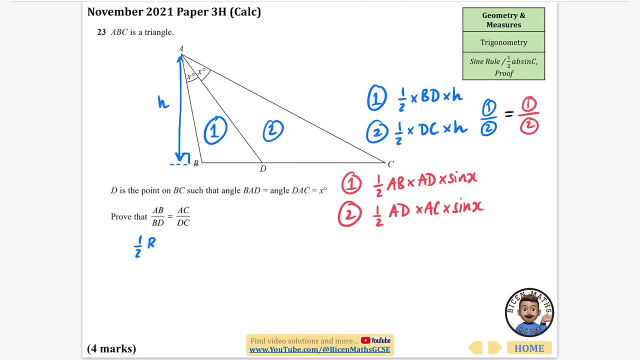 this one. So I'm going to write that down. I'm going to say that my half BD multiplied by H divided by my half DC multiplied by H must be equal to- and this part's in red- my half AB times AD sine X divided by my half AD multiplied by AC. 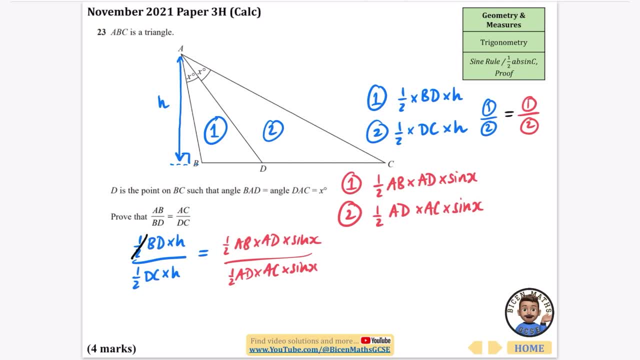 multiplied by sine X. Now the good thing about this is: the half here and here will cancel, the height here and here will cancel, the half here and here will cancel. the sine X will cancel and the AD will cancel, which leaves us with BD over DC equals AB over AC, which is actually very